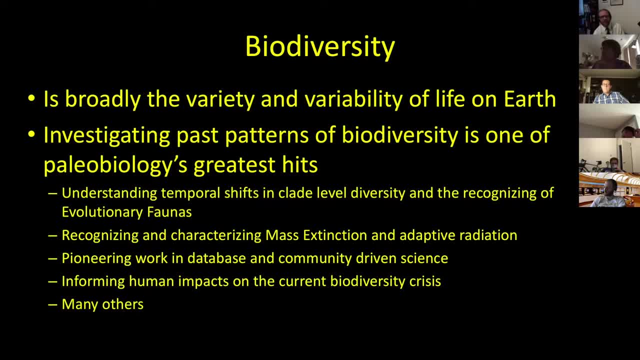 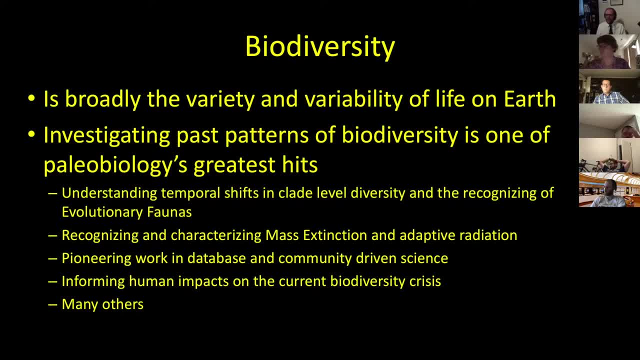 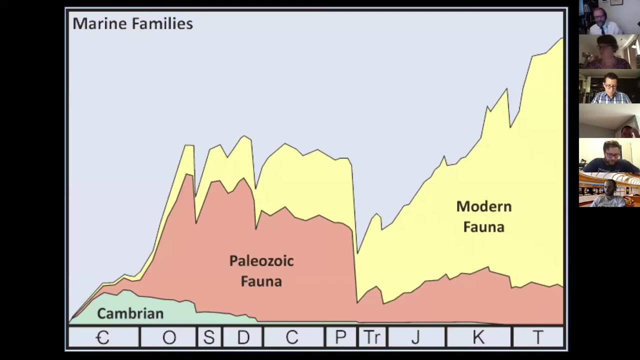 since the 90semeeta and paleobiology that is the curative model. yet You can see in this slide chat part two, which have two global сейчас with the prices: VALIDATES, VALIDATES, ffective VALIDATES, VALIDATES. 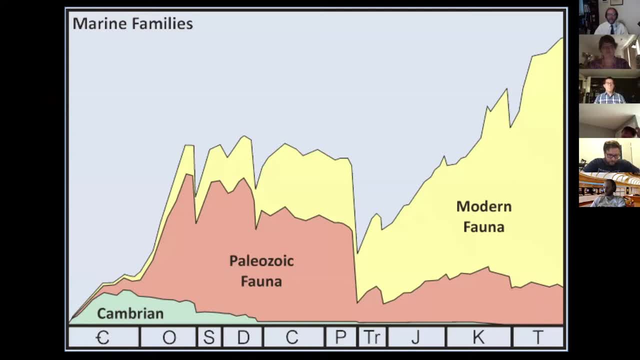 DEFENSE, DEFENSE, EFFECTIVE. old, it's dated, but it is iconic. It's one of the most famous figures ever made in paleobiology And this is nothing more than a histogram, Some measure of diversity along this axis and time here. So things like adaptive radiations go up, extinctions go down, And from that we can. 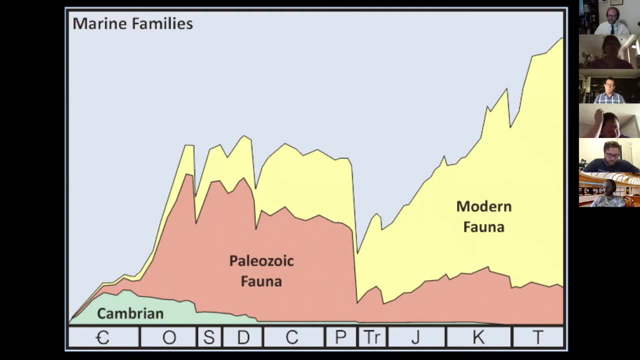 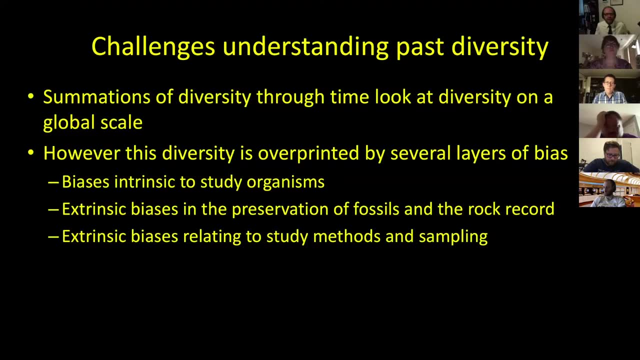 categorize, we can quantify major shifts in the Earth's biosphere. Now, really so. if you think about this, all we're seeing is a measure of biodiversity through time on histogram, But that biodiversity pattern that we see is actually overprinted by lots of biases. 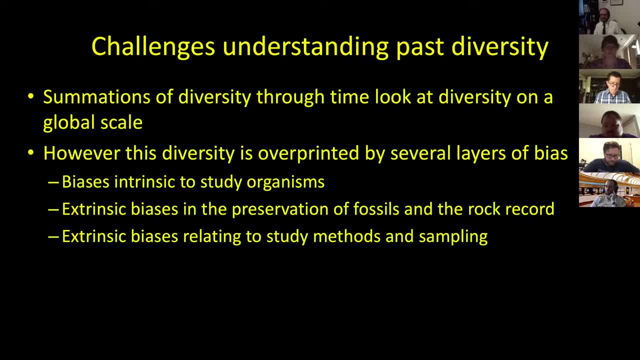 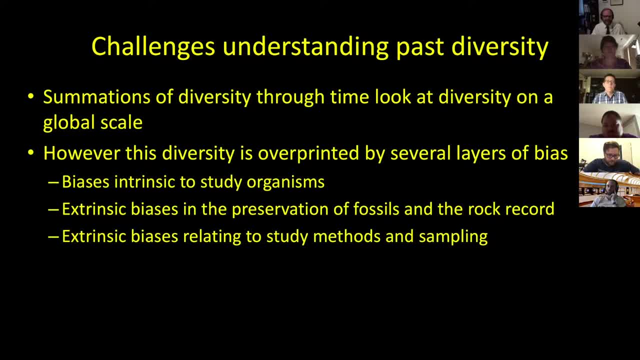 biases in them. But bias is something that fundamentally affects how we understand this, And there are three fundamental different types of biases that I think you can easily identify in these data sets: The bias that's intrinsic to the organisms themselves, something about the biology. 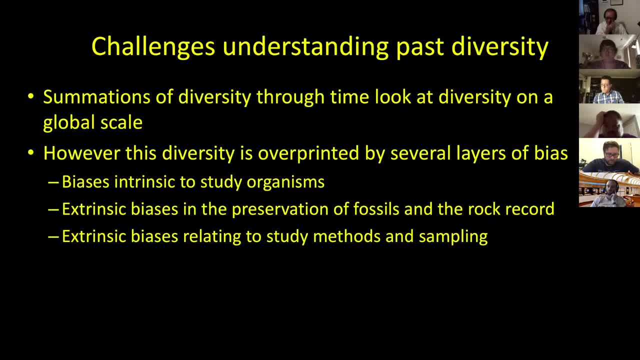 of the organism causes a bias. Biases that are extrinsic to the organism but are the result of some issues with fossil preservation, the rock record, And then, finally, the biases that are associated with the researchers, the study methods, the sampling, 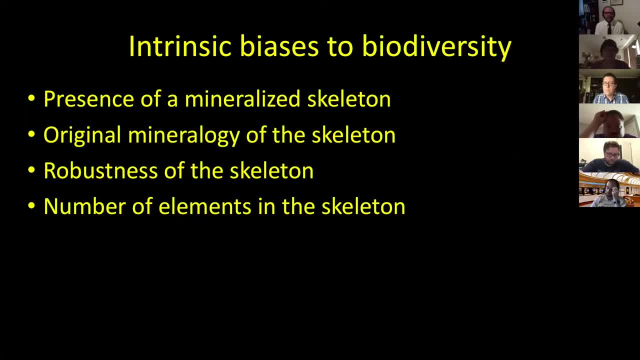 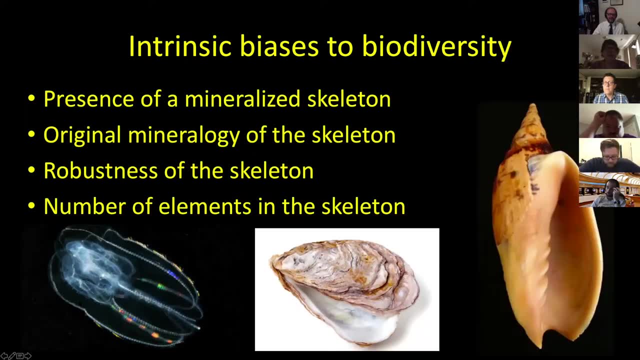 So just quickly to look at these intrinsic biases, might be something like the presence of a skeleton. If you look at these three organisms- a ctenophore, a comb jelly- doesn't have a skeleton, so it's fine. But if you look at these three organisms- a ctenophore, a comb jelly- 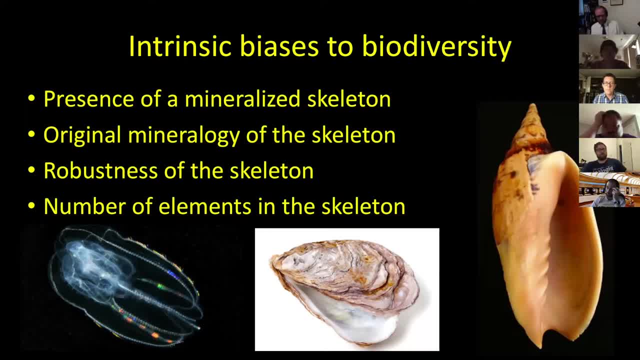 and a swab jelly and maybe a rock jelly, you'd be able to see that the fossil record is automatically in jeopardy. The original mineralogy of the skeleton can be very important. A lot of rocks, like in the Cretaceous, will have both oysters and snails in them. But because oysters are low, 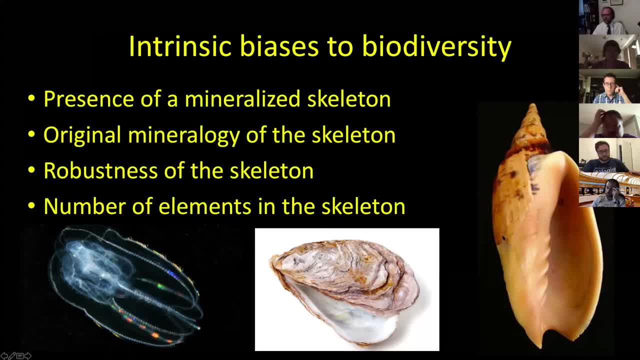 magnesium, calcite, and snails are, generally speaking, aragonite. their preservation potential is very, very different. Oysters are beautiful, snails are moldic. The thickness of skeletons- fragile skeletons are subject to destruction, whereas thicker skeletons are not- And the ability to 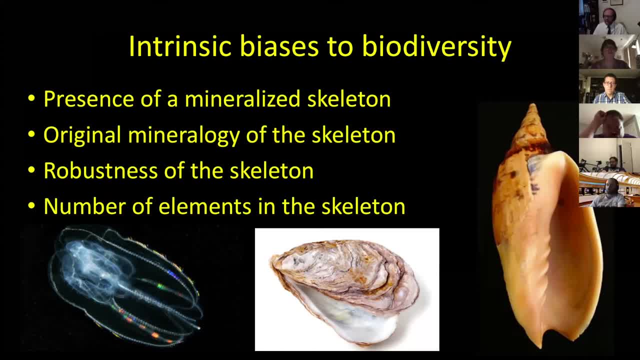 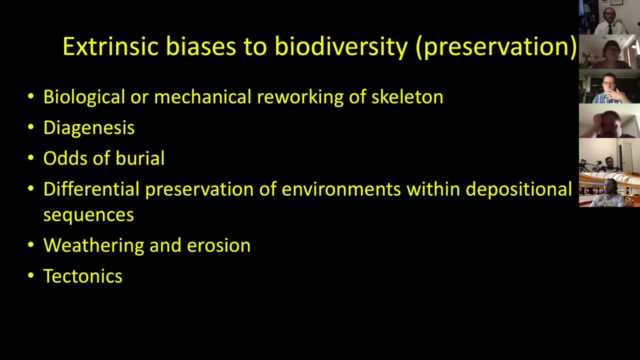 recognize things is often a function of how many skeletal elements they have. Something with a few skeletal elements is good. Something with hundreds to thousands to millions of elements is generally bad. Extrinsic biases in terms of preservation are also a problem, Biological and mechanical. 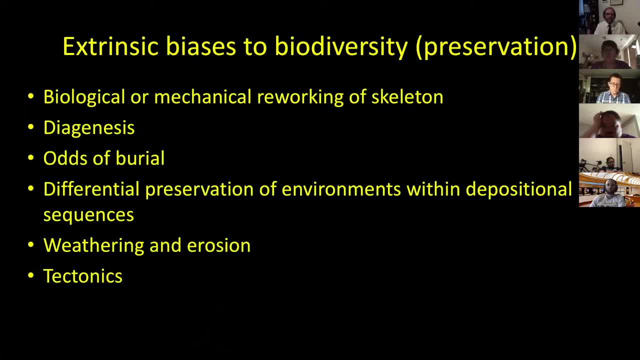 reworking of skeletons, so organisms tearing things apart or being washed down a stream or ground, Diagenesis and other rock processes can destroy fossils or, in some cases, enhance the preservation Odds of burial of organisms. Burial is generally a problem. It's generally required for preservation, But some organisms and where they live and how they 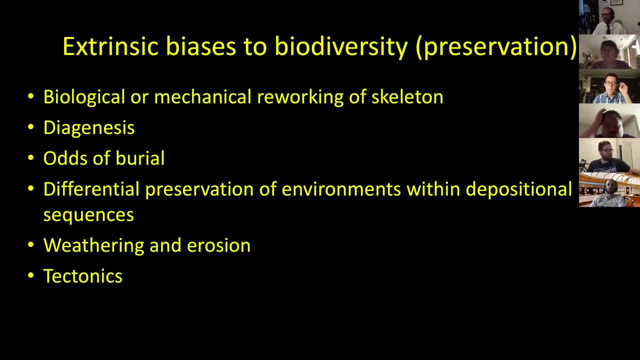 live interacting with the environment are more easily buried than others. Environments that organisms can live in are not evenly preservable within the rock record. Certain types of ecosystems, like high mountain slopes, are never going to be preserved because they're erosional, Whereas places where sediment is being input. 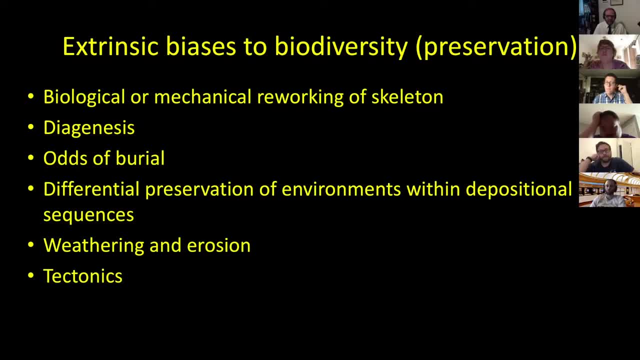 we'll have higher preservation potential. And then we have destructive forces on a massive scale- weathering and erosion and tectonics. So these sorts of things and the previous slide are all things that can fundamentally affect our ability to see fossils and the fossil record. But what's? 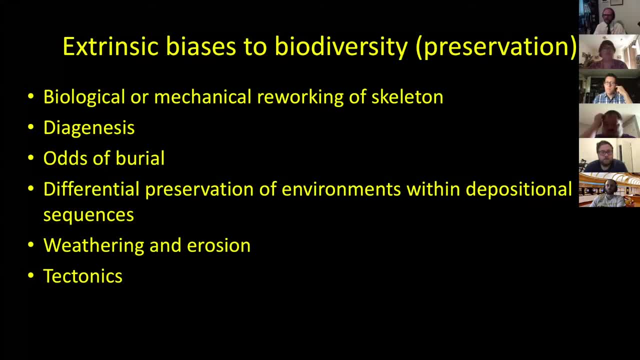 nice about these two categories are we understand them. Because we understand them, we can. we can work with them And we can work with them And we can work with them And we can work with them, We can work with them. We can understand how things are missing And we can mitigate how. 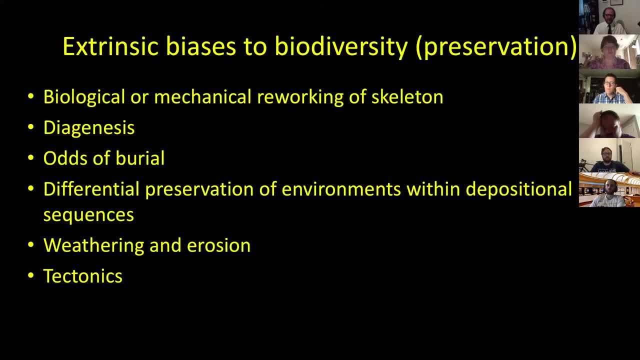 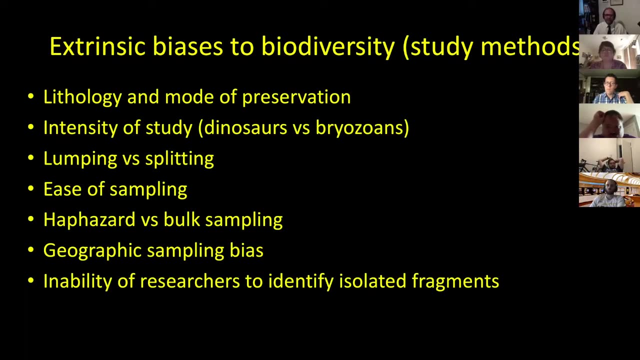 things are missing using, you know, just simple things like I wouldn't expect this. So what do I? what should I expect if I did see it? Where we're much more blind is the biases that are associated with study methods. So the rock that an organism is preserved in, of course, is the rock that the 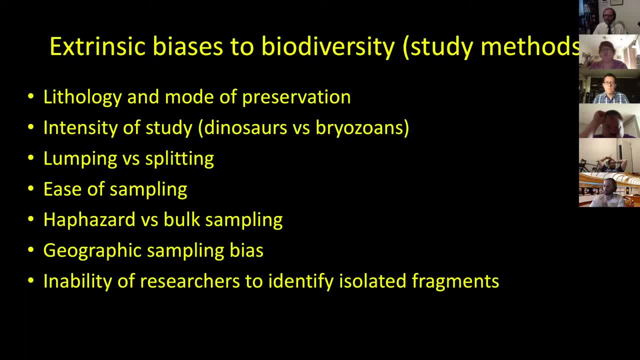 rock that an organism is preserved in, And that's the kind of thing that affects whether or not we collect it, Because certain types of rocks are impossible to get good fossils out of, So we, generally speaking, ignore them. Some organisms, like dinosaurs, people actually study. 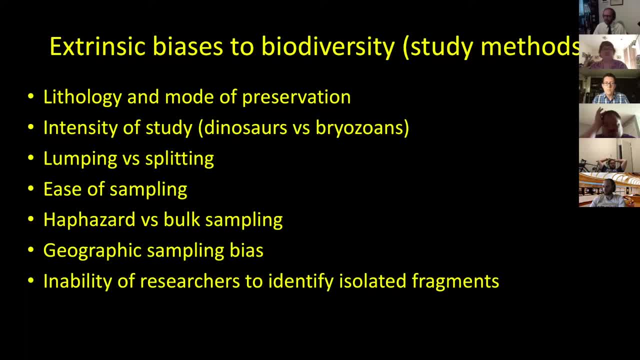 Some things like bryozoans. there's two or three people in the world that look at them And which one makes up more of the rock volume? Well, it's bryozoans by several orders of magnitude. The way we deal with our taxonomy, whether we overgeneralize organisms, 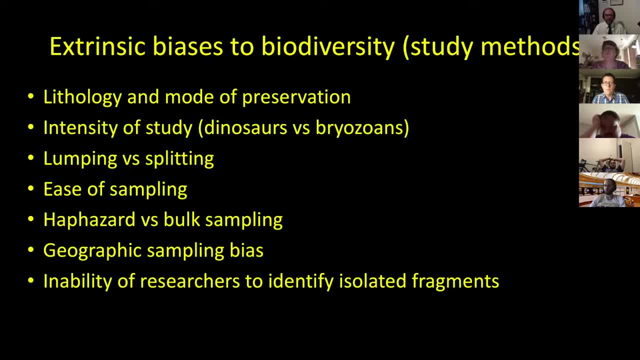 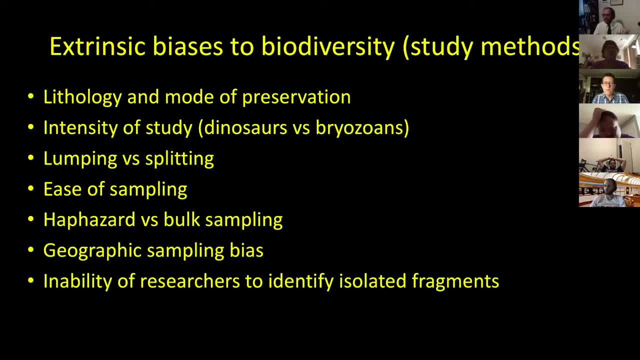 making a single species into numerous species because of of true ignorance of the true nature of things can fundamentally affect our counts, either over counting or under counting. some fossils are not easy to sample because of other conditions. most fossils are haphazardly sampled: we simply walk. 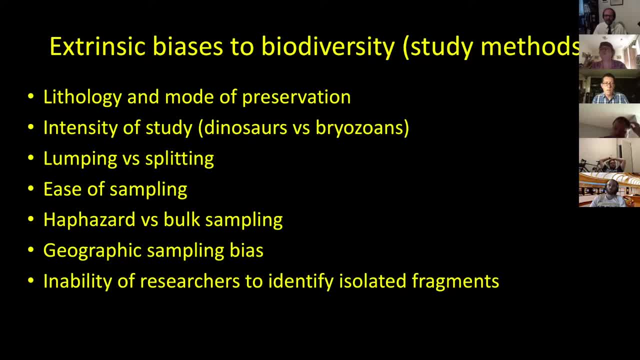 around on our hands and knees picking things up off the ground as opposed to bulk sampling. there's huge biases in terms of geography and where fossils have been found and, very, very importantly, the inability of researchers to identify things that are not complete generally. this requires the experts in the field to look at them and, generally speaking, 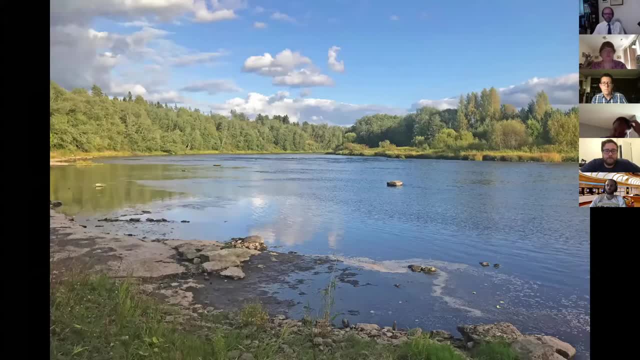 those are few and far between. you might think of it like like this: here's a modern ecosystem outside of st Petersburg, Russia. so I would say, okay, what's the biodiversity here? well, there's several ways you can look at it. let's just simplify things and say animals. well, what do you mean, do you? 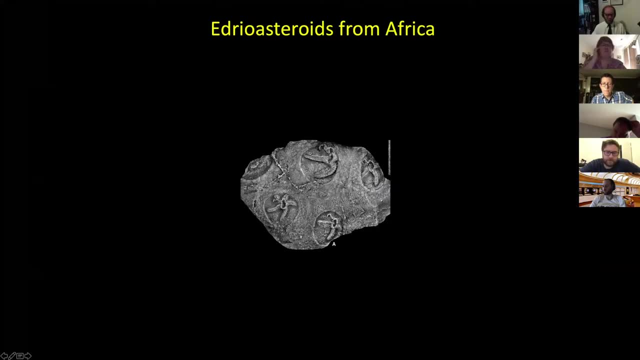 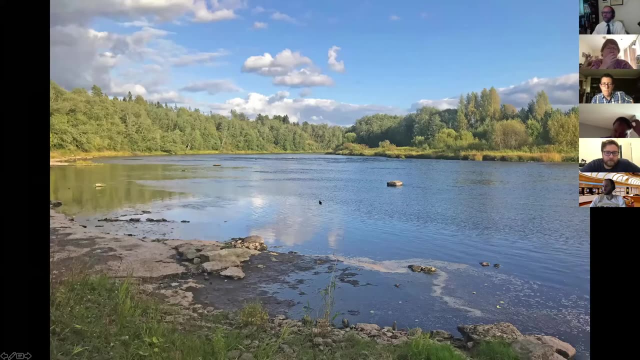 mean the animals that live in the trees, the animals, oh, the animals- that live in the mud flat, the animals that live in the water. those are different things and maybe your, your research methods, will pick one of them, or maybe it's something like: are you talking about the animals that are? 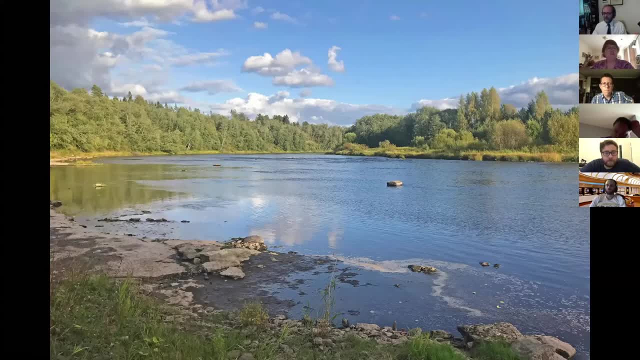 diurnal animals, ones that are active in the daytime versus ones that are active at night, common animals, rare animals- the way you sample this can fundamentally affect how you perceive that ecosystem, and that is also very true in the fossil record, because the same sorts of things happen- not not these exact things, but it's a lot of decision. 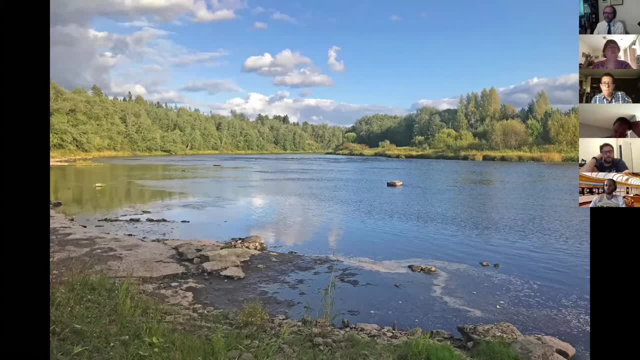 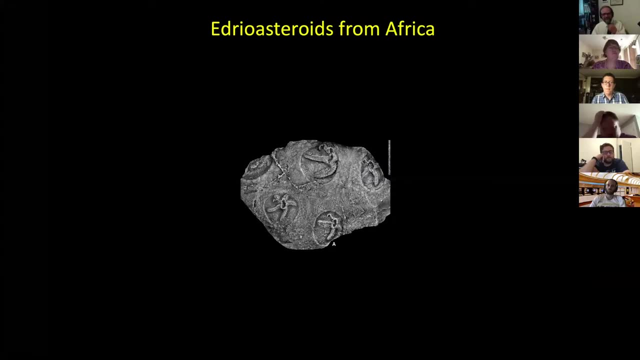 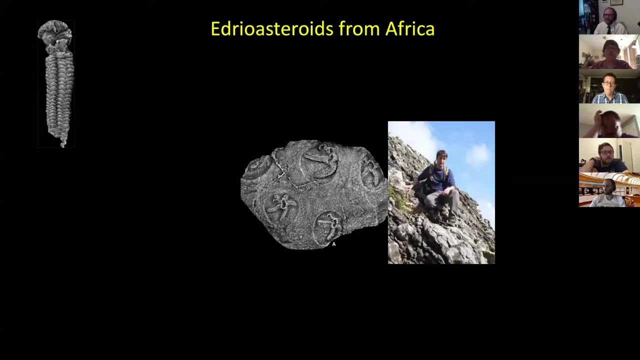 making on what you collect, where you collect, how you collect, will change the way you perceive that biodiversity sampling bias also shows up in geography in 2008. this is the exact degrees of können and a you ic. Can go on for a while. each preserve One thing. i find things like that. last course it lift and sample the size of theOSHI. do it like here. you get a mental issue. but this ideal architecture changing said that we need the logic that the fossil sand had. theЛah gay кол-sat or zone brewhomér meant that the fossil's time they were quarrel industries at the bin, just to top rectored in AEM or megabas. you've 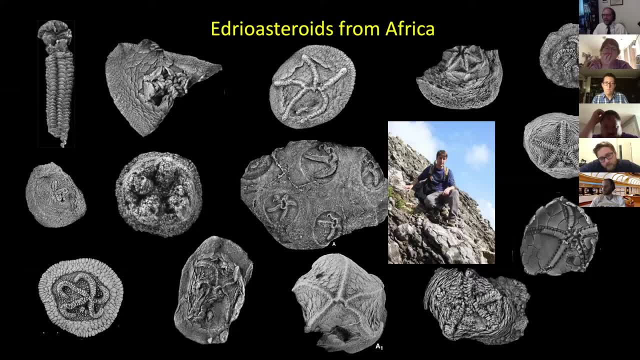 hours. He found all those species of Eadreo asteroids in an area about the size of Knoxville. Why is that? Because no one had looked. So now the the Eadreo asteroid fauna of Africa is as diverse as the fauna of the Ordovician of the mid-continent US. 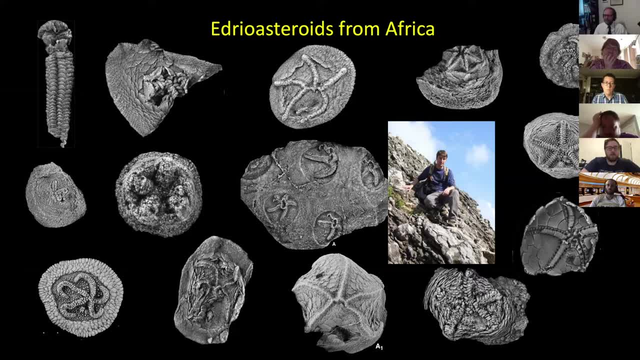 But we didn't know that until it was actually sampled, And the environments that they occur in are fundamentally different. Eadreo asteroids prior to this work were assumed to be tropical living in carbonate environments. These were sitting on the south pole, 89 degrees south. 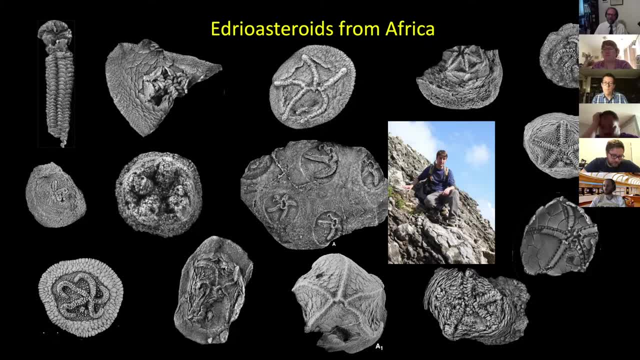 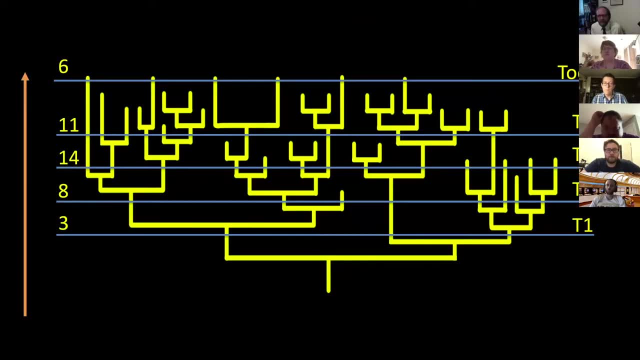 in siliciclastics very different environments, So that sampling bias fundamentally affected the way we see things. We also have biases that are associated with the fact that we're dealing with fossils. Now, one thing that's true about fossils is, if you have a tree of life- and this is just 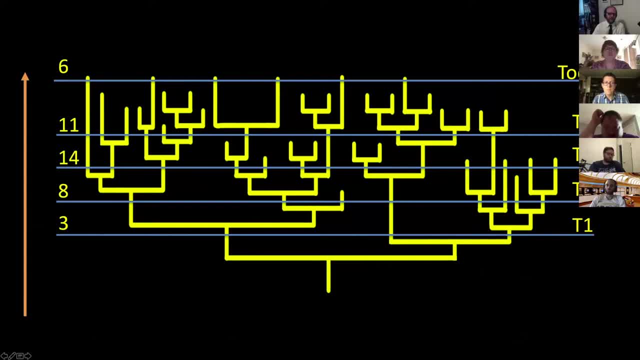 you know a diagram of an evolutionary tree and time goes up. if you sample this at different time intervals and you have good sampling, you will see that there's a pattern of diversity. At this timeline- the lowest one time one- we have three fossils. Here we have eight. Next one, we have 14.. The next one, we have 11.. 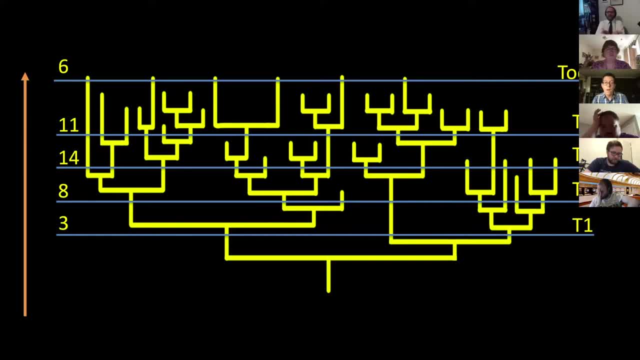 The next one, we have six. So the diversity expanded and then contracted. If you don't have a fossil record, you get a fundamentally different pattern every single time. If you go top down using the tools of biology like genetic data and things like that, 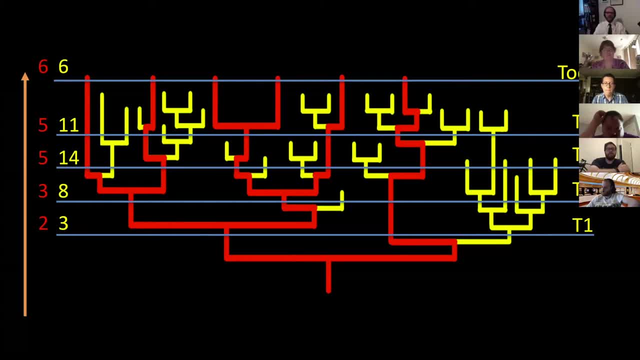 you will only see an inverted cone of diversity, because the lineages that are highlighted in red and red are visible from a top-down view and the ones that are highlighted in yellow are invisible to that toolbox. And so, whereas here in yellow, over here we have expansion and contraction of 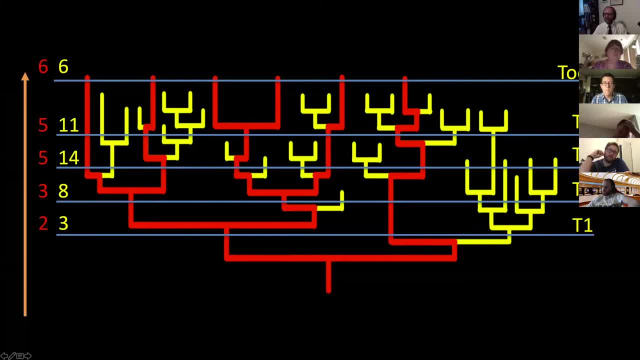 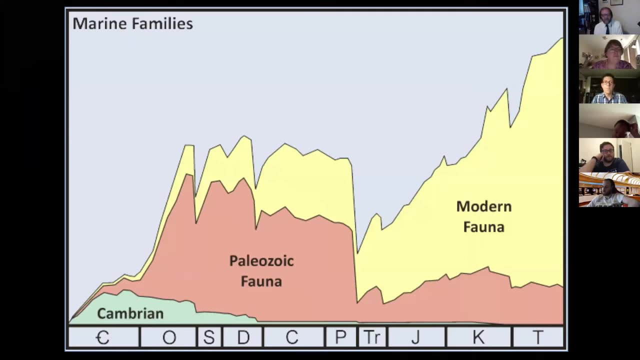 biodiversity. here we have increasing biodiversity, So that fundamentally changes things, and this is actually one of the main reasons a fossil record is important to study. So with all of that, we have to address a few questions. Is this pattern robust enough that the way we sample is not influencing the way this pattern is perceived? 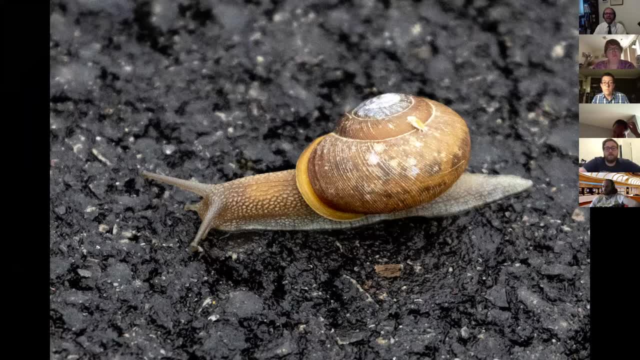 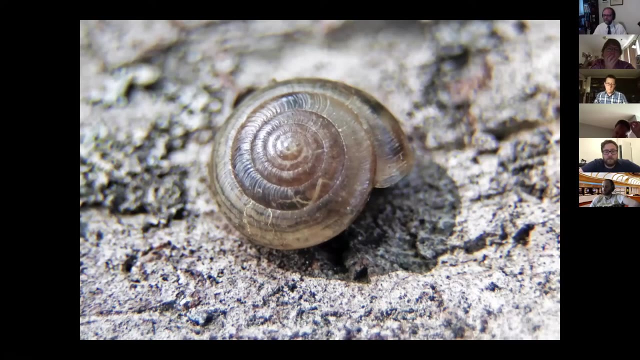 So I'm going to talk to you about a group of organisms that has a bit of a checkered history in terms of its preservation. If you think about a thing like a snail, this is a snail. if it dies, how many parts are left? One right, Simple enough. and if you saw a snail, 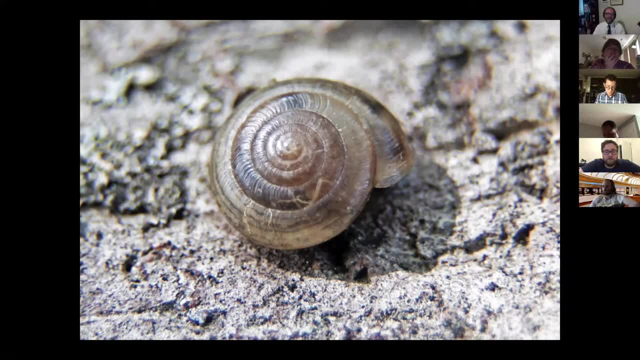 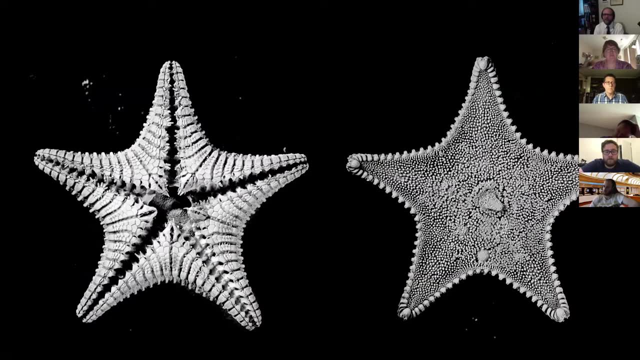 shell, you would say, oh, a snail. It's not rocket science, This is an echinoderm, It's a starfish. I would argue that this animal has a few more than one part, A few different counts. you do do. most echinoderms have between 10,000 and a couple of million parts, And most of them. 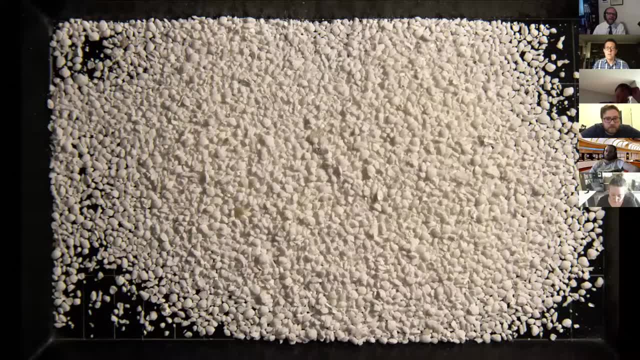 are ridiculously tiny When they die. this is what they turn into. This is a starfish soaked overnight in bleach, And the human mind is very good at simplifying, and the way you simplify this is you call this sand, And when you call it sand, it goes away. 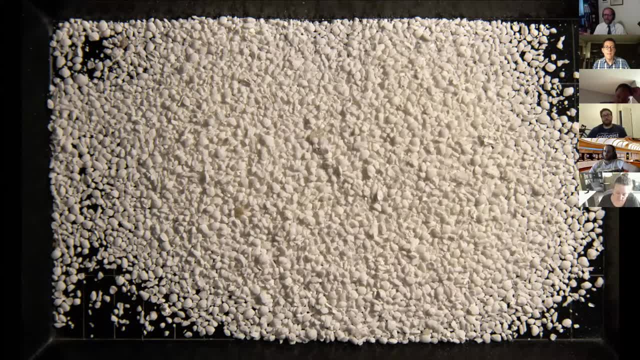 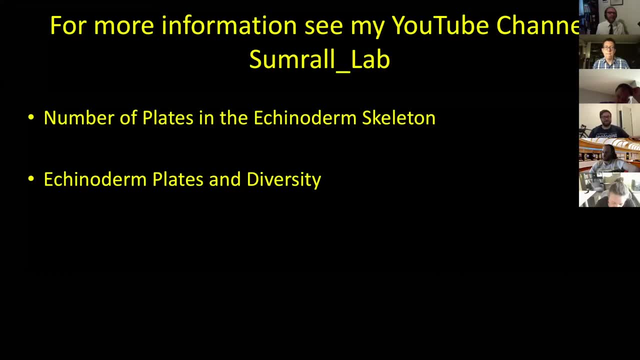 And if you looked at this, there are only a handful of people on Earth that could make any sense of this as anything other than echinoderm hash. If you want to know more about this, I've actually made a couple videos on my YouTube. 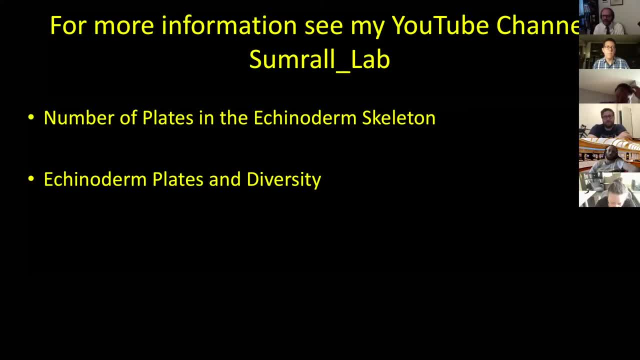 channel about this, so just drop by and you can see. Those are the two videos that relate to this. How many plates does an echinoderm have, where I have a time-lapse video of an echinoderm exploding, which is fun, And just another video there, Anyway. 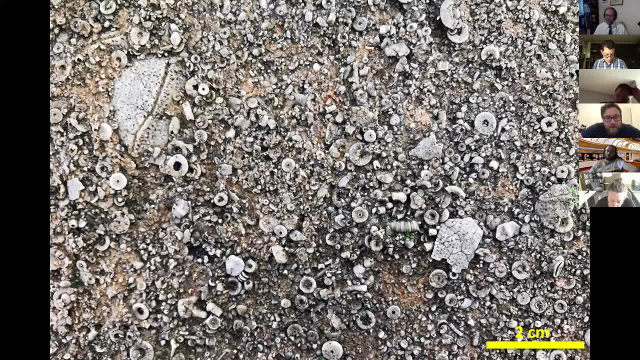 So this is what echinoderms almost always look like in the fossil record. This is called an encrinite. The name comes from the fact that it is a whole bunch of crinoids, And I think everybody knows what a crinoid looks like. You know poker chips with a hole in it, right? 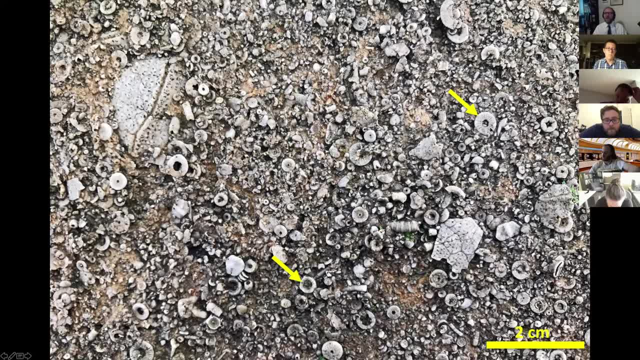 But even a cursory glance, I'm hoping that you can see that you know this crinoid has a circular hole. This one has a pentagonal or star-shaped hole. This one has a pinhole. This one the hole. 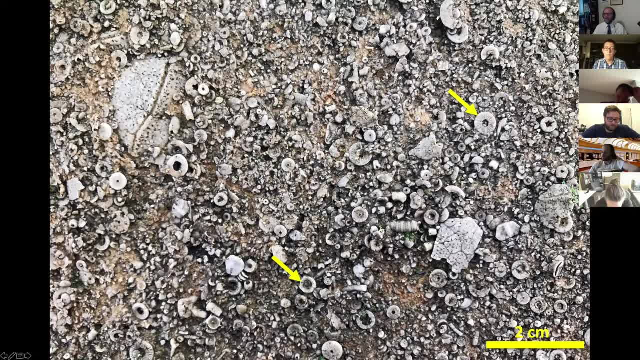 has a lip on it. There's a lot of different kinds of crinoids in here. So if you just say crinoid, it makes it sound like a crinoid. It doesn't sound like your diversity is one species of crinoid, when really it's a lot. 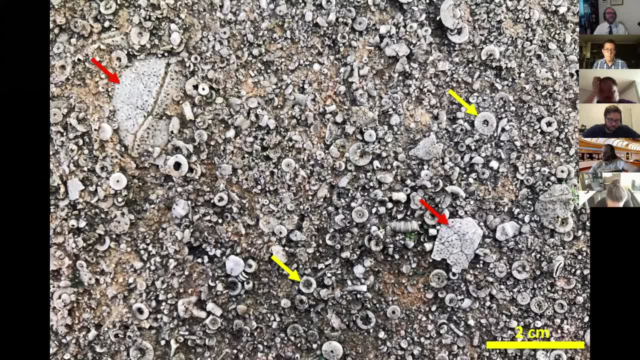 If you look harder, you can see things like this. This is a diplopyrite. These were last looked at in our department by Sarah Sheffield And again, it's something that not a lot of people would jump out at. And over here we have plates of a rhombiferin. 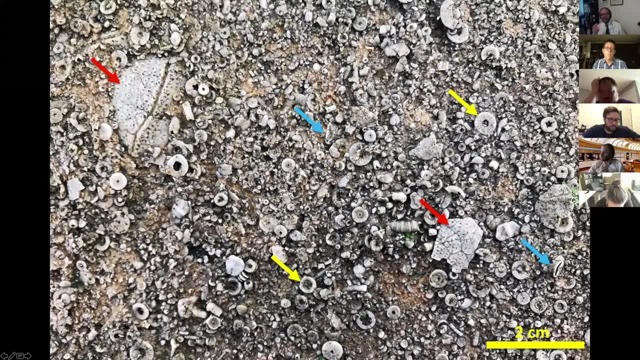 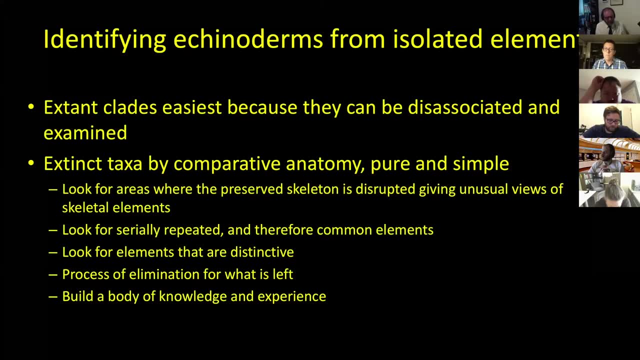 There's also blastoid plates, And if we put this under a microscope, I'm sure we can find a lot more things. But you really have to know what you're looking at in order to make any sense of this. So it's not a simple process. So what I'm going to argue is: you can actually identify these elements. 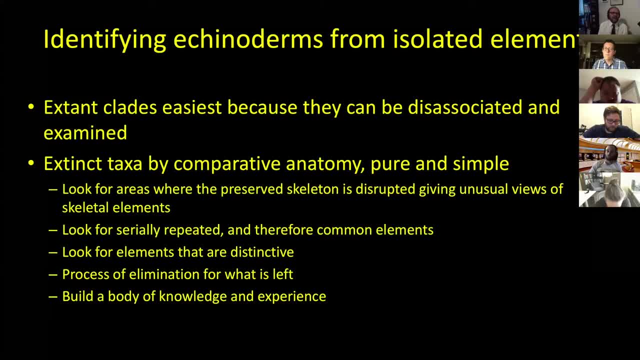 if you know what you're doing And the way you do. this is actually fairly simple. If it's an organism that's alive today, you can simply disassociate one, And then you understand what the parts are, because you have them loose and free and you can look at. 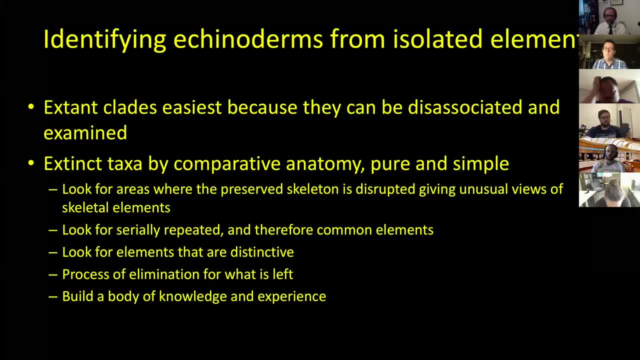 them at your leisure. If they're an extinct group, it's a little more complicated. You have to use some very careful comparative anatomy. You look for specimens that are well-preserved, except for an area that are disrupted, where you get things jumbled, so you see different angles at things. 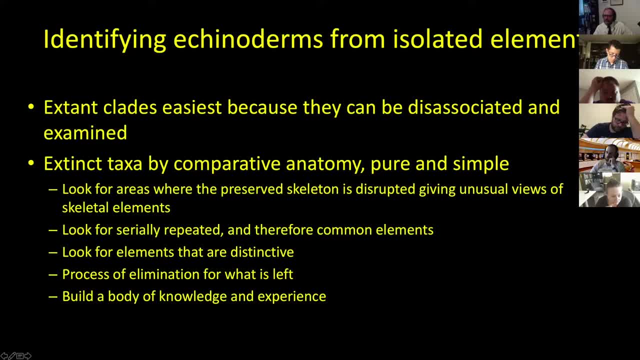 You look for elements that are serially repeated. Serially repeated elements are common, and so you're more likely to find them in a pile of hash. You look for elements that have something very distinctive about them, And what's left? you work out with a process of elimination while building a body of knowledge. 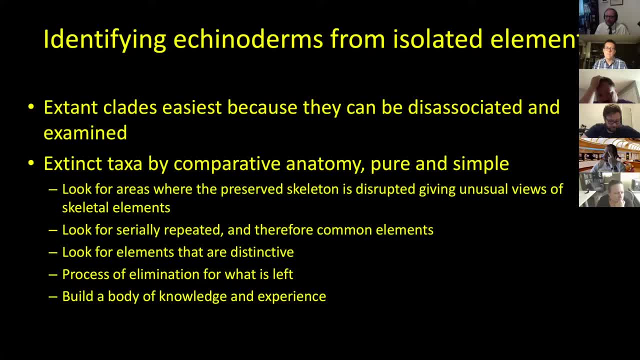 and experience. I can tell you from my personal experiences working with students that there's a pretty steep learning curve, but once you get there, you're. it's really amazing how quickly you can actually identify different types of parts just through having seen a bunch of them. 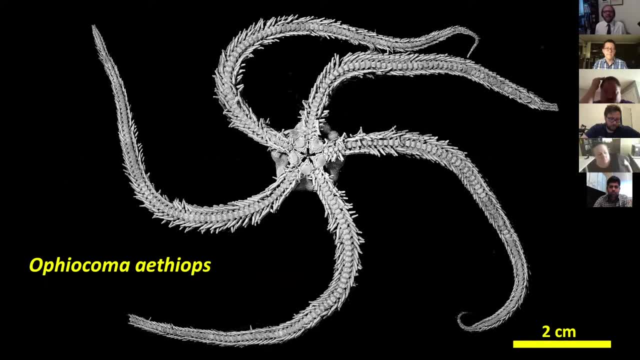 So this is, this is a brittle star, and this is just an example of how we look at something. Obviously, this thing has, I don't know- 10,000 parts. let's say So how do you deal with it? 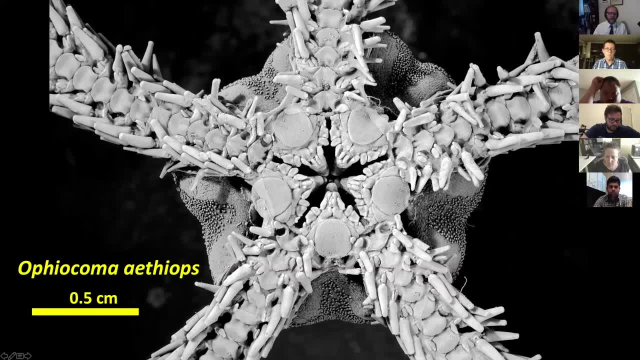 Well, if you go in and look at the mouth, what you see right off is there's lots of plates. In fact, most of the plates are these little tiny platelets over here. There's no way you'd ever be able to know what those are. They're just small. 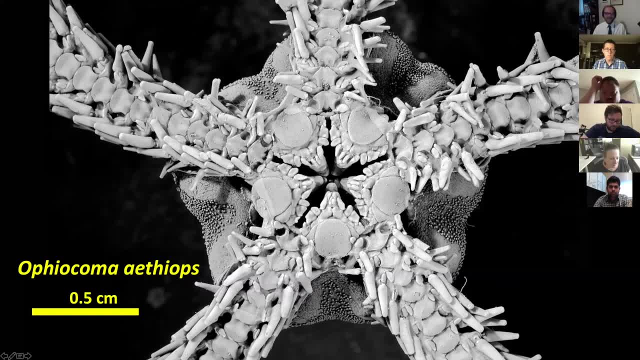 nondescript little plates that are, you know, 50 microns across. There's plates in the mouth area that are very distinctive. These plates right here, for example, are very distinctive. There's 10 of them on the whole animal, And so you're dealing. 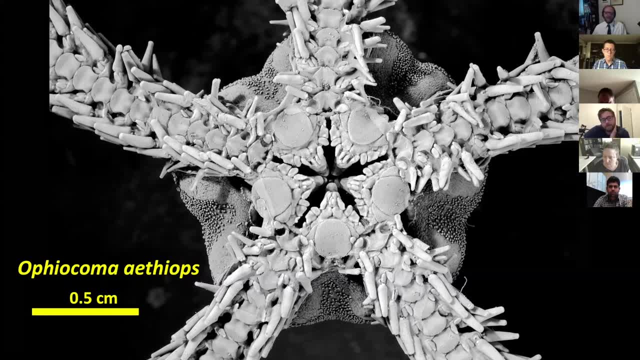 with 10 plates out of, let's say, 10,000. So you're going to have a hard time finding them. If you go to the top side of the animal, you know you don't have a lot of help there. You just got a whole bunch of stuff. 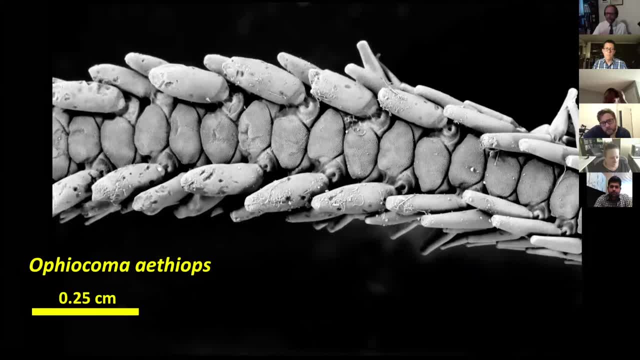 But now let's look at the arm itself. The arm is a whole series of serially repeated segments. Because of that, we have a series of plates here like these. These are called dorsal shield elements and they they right and left, but they're orderly and understandable. We have these plates here. 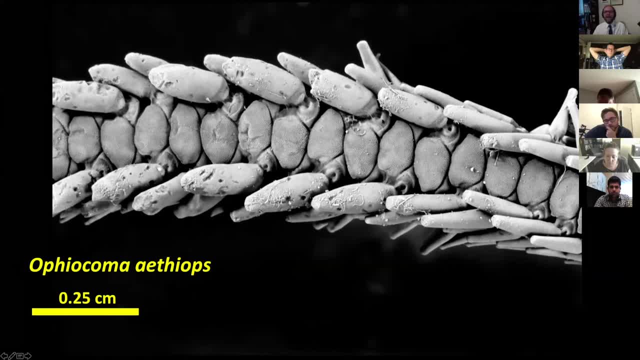 with the spine bases on them here, here and here, and that's called a lateral arm plate. Again, those plates serially repeat, so we have a lot of them and because of that we also. they're orderly and understandable. They're also very 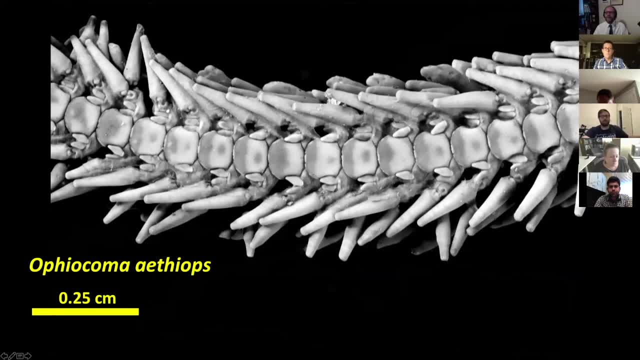 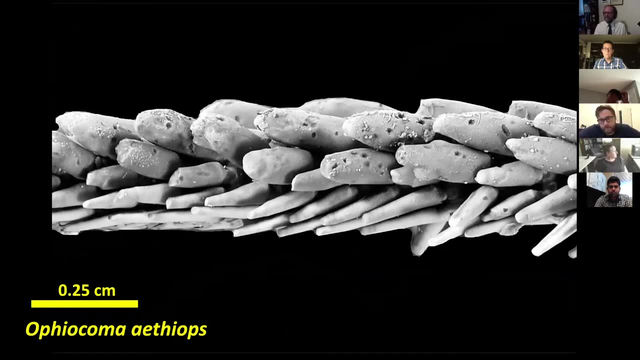 distinctive. The bottom here's our ventral shield plates, a lot of things that look the same, but again common, and the spines again orderly, but not distinctive in any way. So the bottom line is, when you look for parts of an 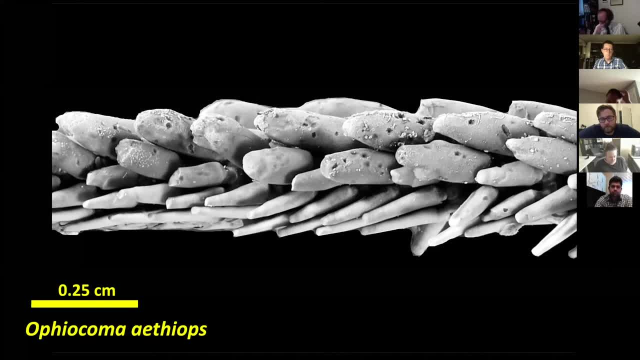 animal like this. research has shown in the Mesozoic that the primary plate you're looking for are the long-tailprofit and the long-taileds, which is where the lateral arm plates, where the spines attach, and the plates that core the center of the arm called. 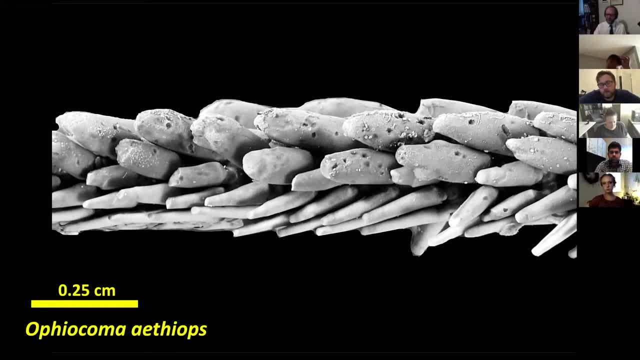 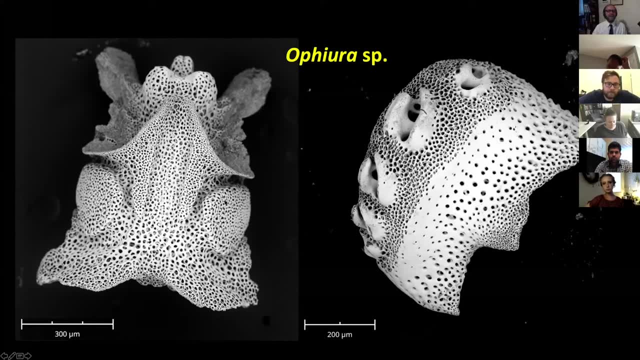 the vertebrae. Those plates are distinctive and we can understand them. They look like this: This is a vertebra element. All these holes- that's the microstructure of them. That's what they look like, because those are full of the soft tissues. This is one of the lateral arm plates. 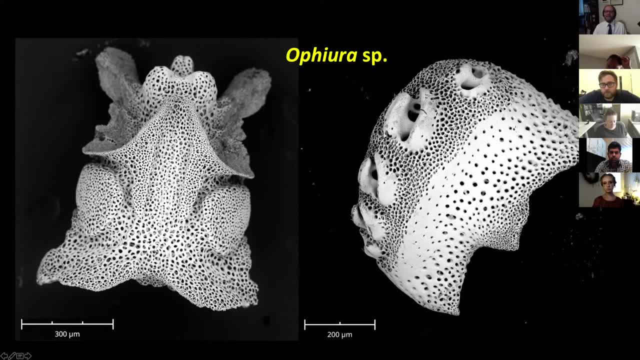 Look at all the morphology here You have these. you can count the number of spine bases. The spine bases have some interesting sculpture, different pores, that things come in and out of different types of microstructure where the plates overlap each other or form the body wall. So there's a lot. 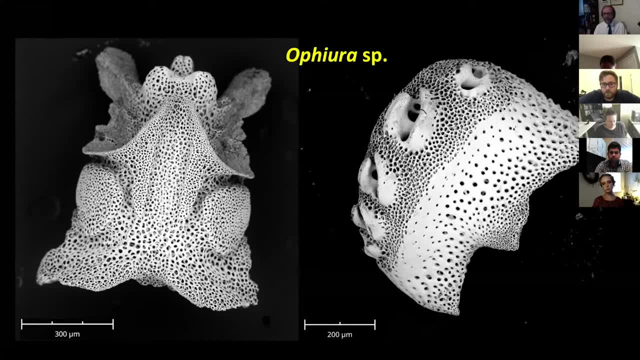 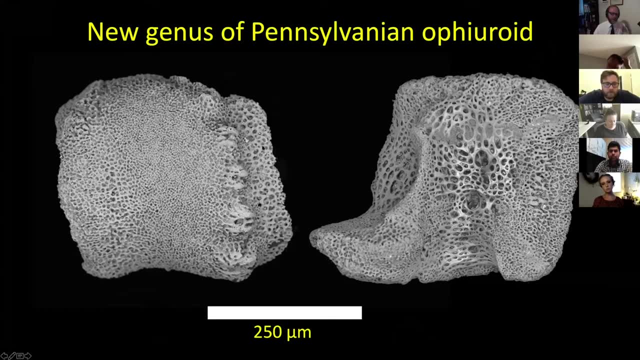 going on here that you can learn from And because we can understand these. in the modern, we can find the same things in the past. This is a Pennsylvanian form. Here are the spine bases, These are the spines, These are the vertebrae. These are the vertebrae, These are the. 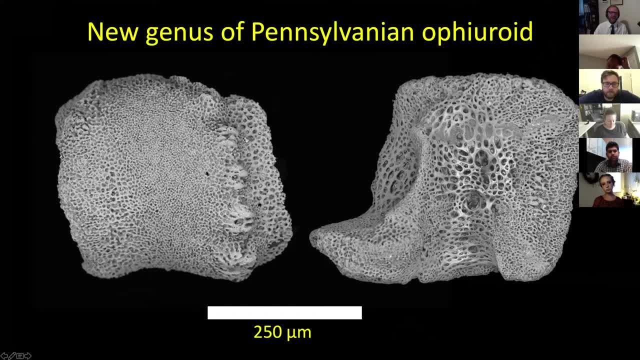 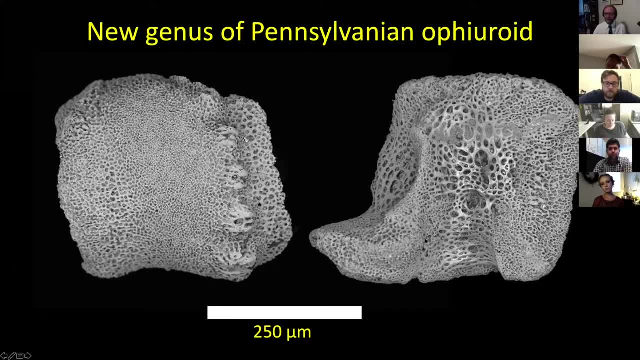 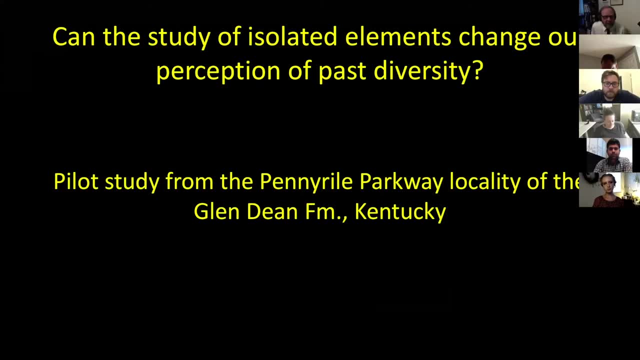 these are beautiful. This is the kind of thing you just die to see. Okay, So I've put up the straw man that isolated plates can change our perception of biodiversity. So what we're going to do now is we're going to go to a. 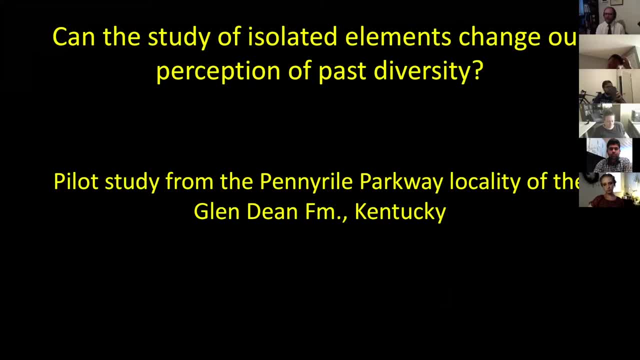 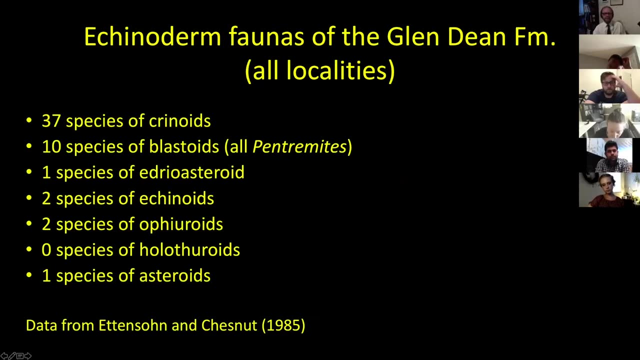 single locality and see how that single locality, based on how you sample it, will fundamentally change our perceptions of biodiversity at different scales. This locality is in the Glendene Formation, which is upper Mississippian. That locality, or the Glendene Formation, has been 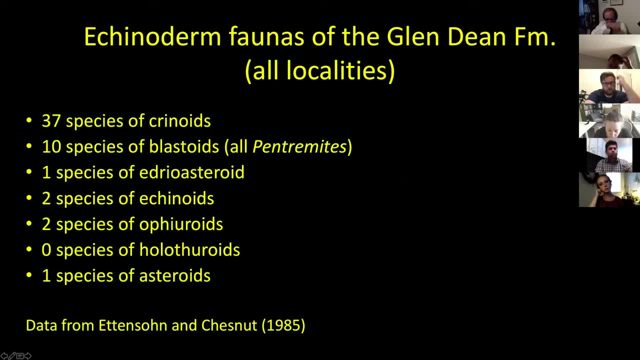 studied from countless localities all over the state of Kentucky And we're going to go to a, And a summary from Chesnut suggests that they are 37 species of crinoids, 10 species of blastoids, one species of edrio asteroid, two sea urchins, two brittle stars and a starfish. 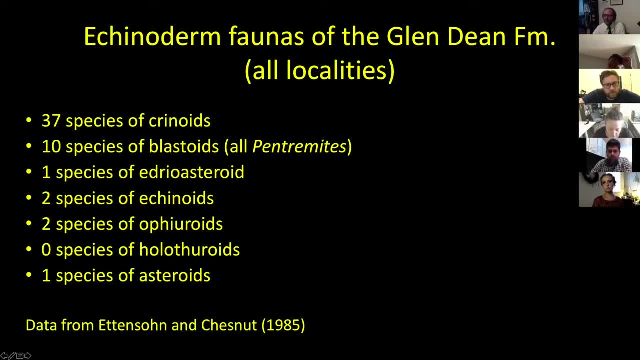 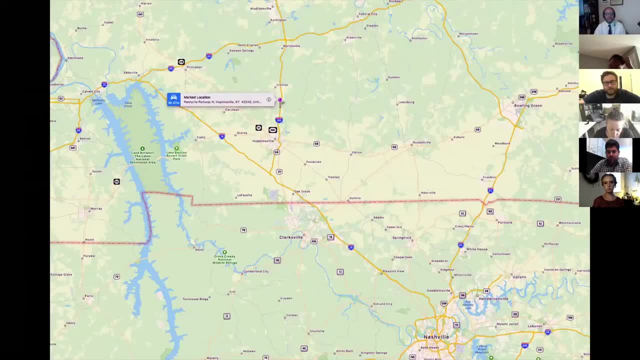 These are all from whole specimen data, so people going out finding a slab of rock with one of these animals stuck to it, We're going to go to a little road cut right here north of Hopkinsville, Kentucky. So here's Nashville. this is up here. 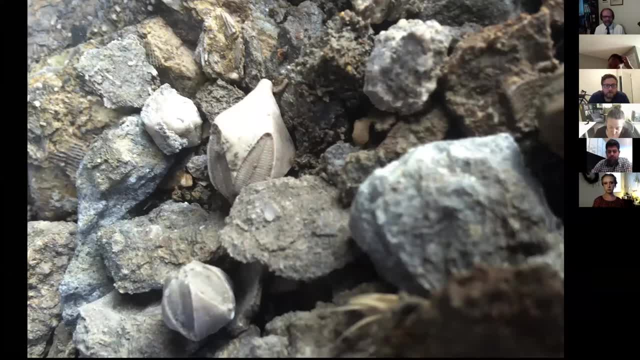 To say that this locality is full of blastoids is an understatement. In this picture there's three blastoids just sitting on the ground. You can go out there with five of your close friends and leave with 2,000 blastoids in an hour. 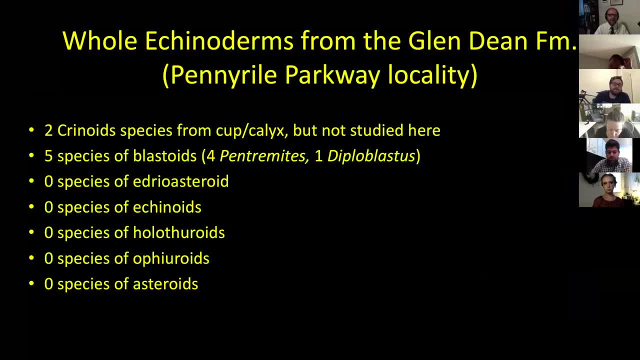 It's that dense. I've been there maybe five times with students. on all these occasions We probably spent about 30 man hours going over this road cut. And this is the echinoderm fauna we found in this road cut: Two species of crinoids, five species of blastoids, including one. 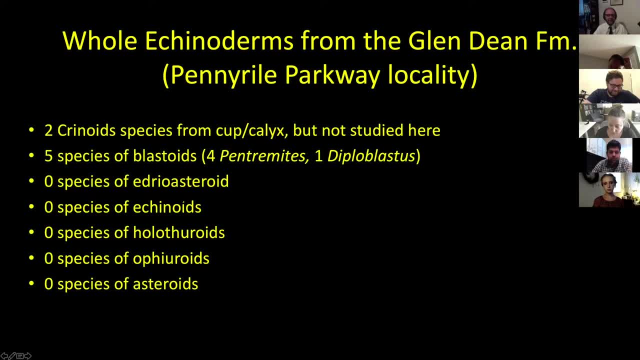 that Chestnut, and Edison didn't have Nothing else. So from this perspective we can say: wow, this locality's got an awful lot of crinoids in it or blastoids in it, and not much else. Here's the road cut. 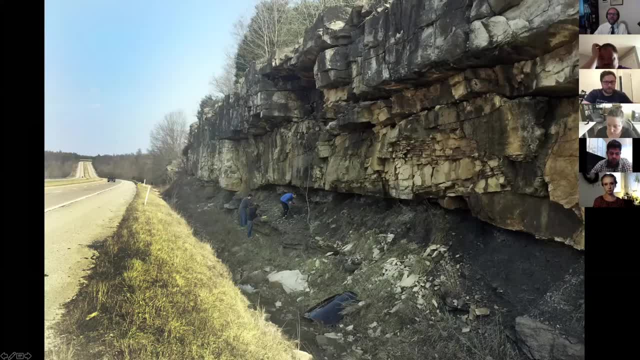 This shale unit is where all the fossils are coming from. This is a Neolithic shoal up here, Beautiful, beautiful grain, And you just walk around and you pick up things, You move the car doors around as need be and, you know, collect your fossils away. 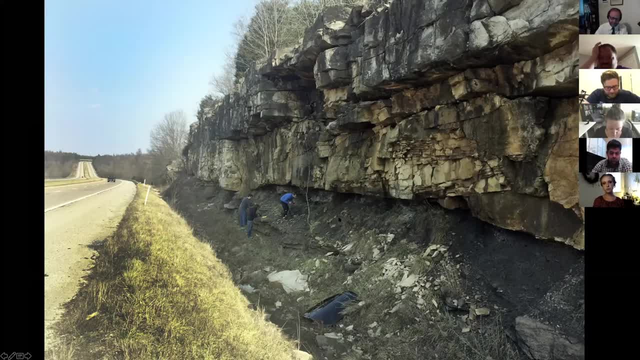 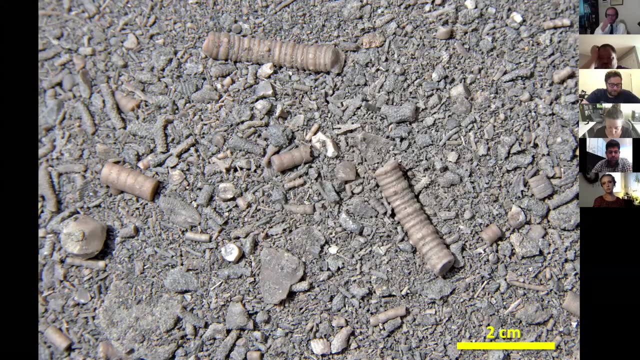 And, like I said, it's just amazing how many fossils are here Now. we surface collected, but we also brought back bulk samples. You wash out the bulk samples and this is what you get when you wash all the clay out. So all of this, every bit of it, is a fossil. 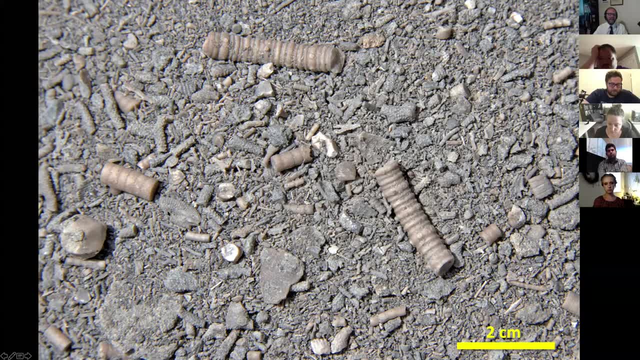 It's a fossil grain, Crinoid here. blastoid part here. Here's a whole blastoid bryozoans, whole nine yards. So rich, diverse fauna. The problem is you can't look through that because it drives you crazy, because the big 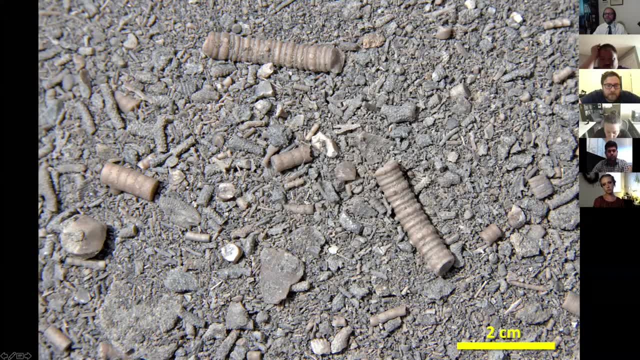 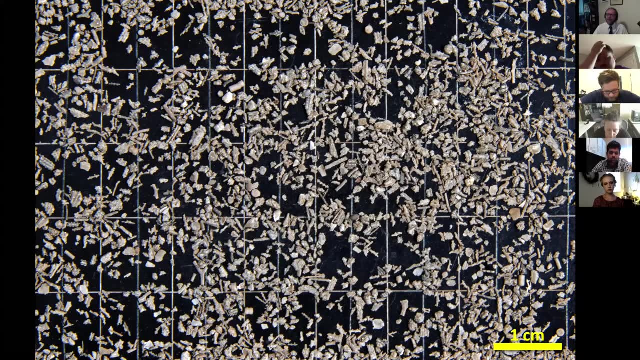 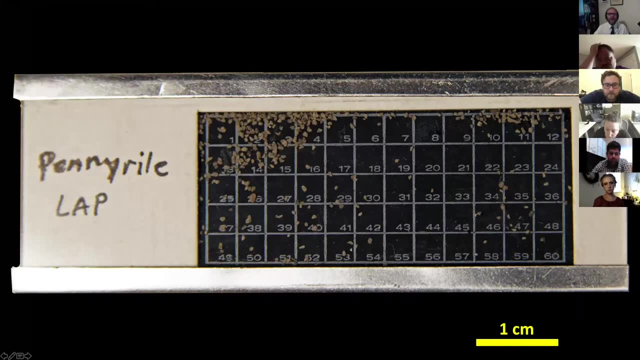 things make it hard to look for little things, So you have to sieve it out, and when you sieve it it looks like that, And then you simply go through that material under the microscope, picking material by hand, and you wind up with little slides covered with very exciting, if you care, echinoderm. 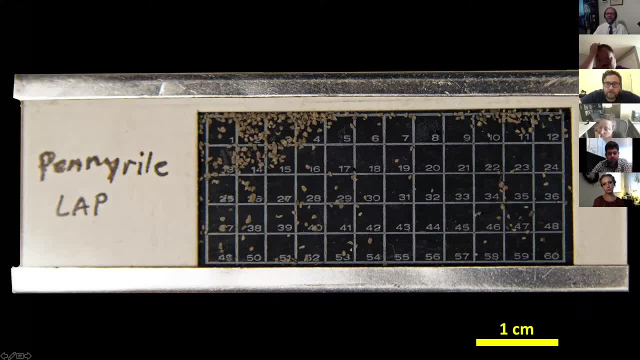 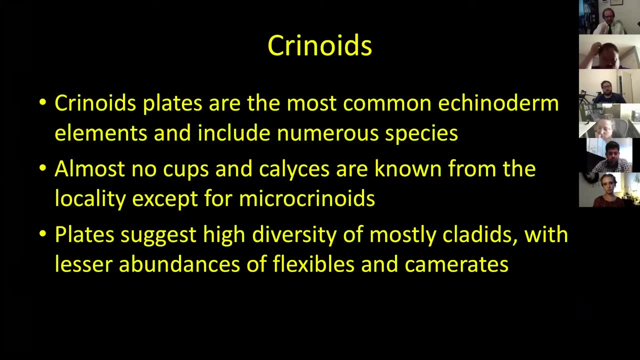 parts okay. So it's a long process to get here, but you wind up with an awful lot of material at the end of the day. So the crinoids at this locality are the most common echinoderm element. I am not a crinoid worker. 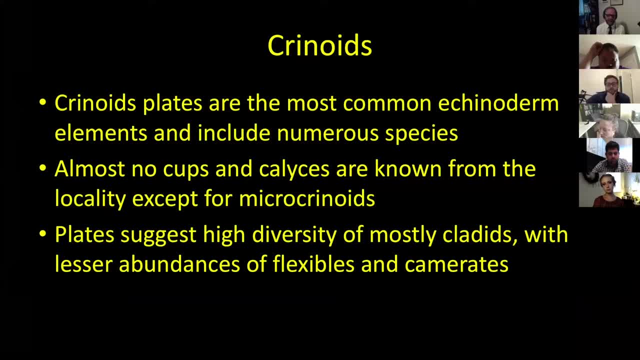 So I cannot say anything terribly useful about the crinoids. From whole specimens we only found two species, But there are lots and lots of different kinds of plates at this locality that I couldn't actually identify. Mississippian crinoids at this time are among the most challenging crinoids when you have 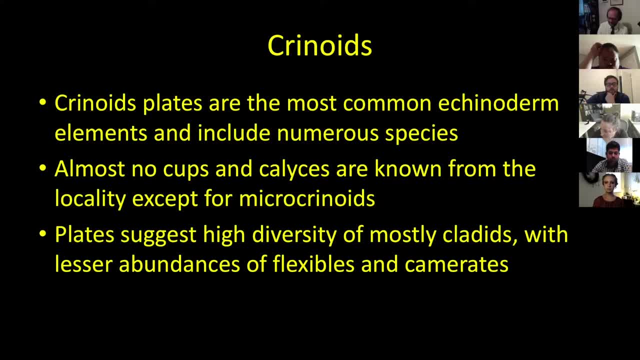 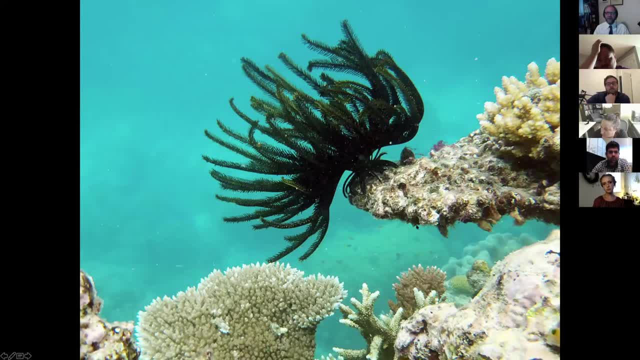 whole ones, And having isolated fragments is really a specialist's job, not mine. For those of you who don't know what a crinoid is, it's a very complex, very complex, very complex crinoid. Here's a modern crinoid in the Great Barrier Reef. 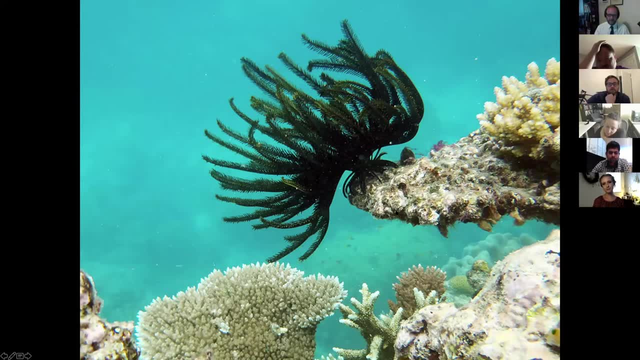 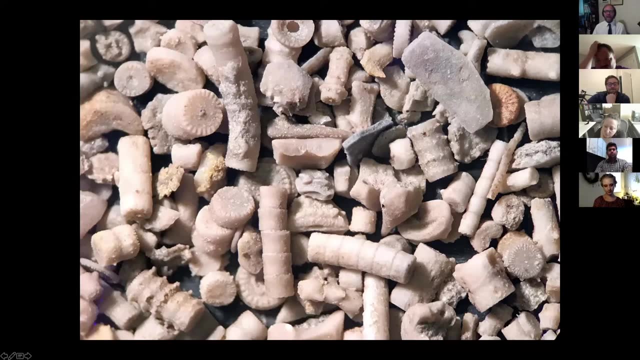 It was so cute sitting there. But we see that And again, you know, even not knowing a lot about crinoids, I'm sure you can see that this stem is very, very different from this stem. This stem is very different. 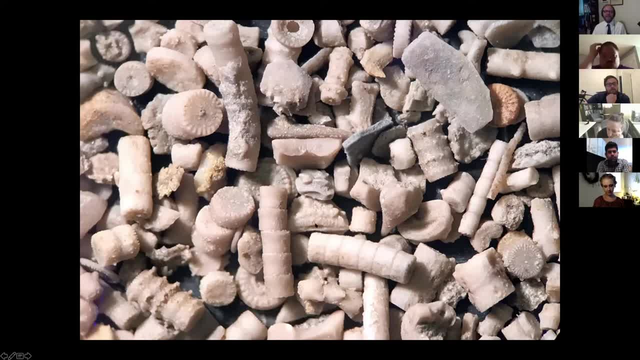 This stem is very different. And then these are plates of the body of the calyx. Oh, these little bits here: arm elements. We got the whole animal. It's just a mess And I'm not going to. I can't put a number on this. 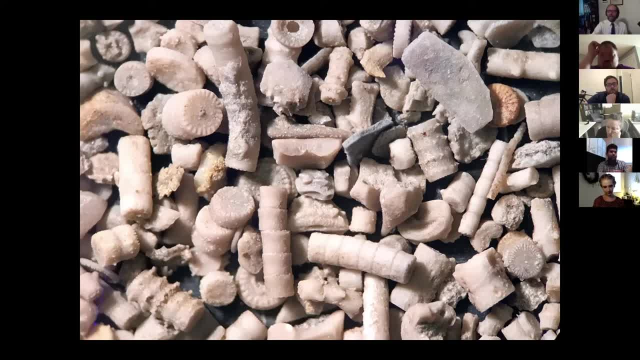 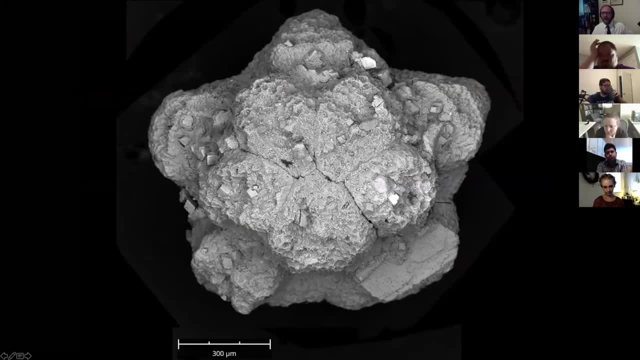 I don't have that skill set, But from what I see here, there's certainly lots of things. What we can add to the fauna are microcrinoids. This is a group of crinoids that are only a millimeter high when they're mature. 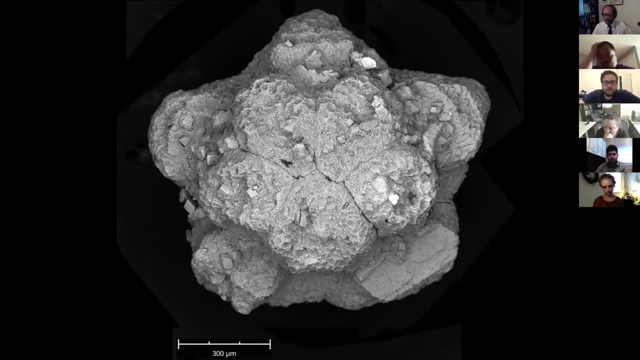 And we see lots and lots of these. So this is something, again, you wouldn't see just crawling around in your hands and knees, Although I had a student once pick one of these up in Texas. Seriously, they just go, poof and picked up a fossil that was a millimeter across off. 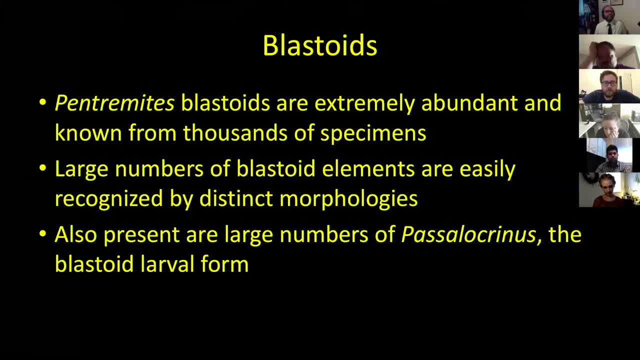 the outcrop Blastoids. Again, blastoids are extremely abundant here, literally thousands of them. But the nice thing is is we understand the morphology of a blastoid, So it's relatively easy to pick them up. What's also present in huge numbers are larval blastoids, what's called Pasilocrinus. 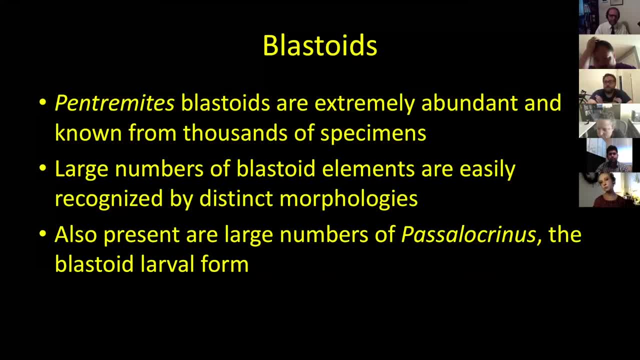 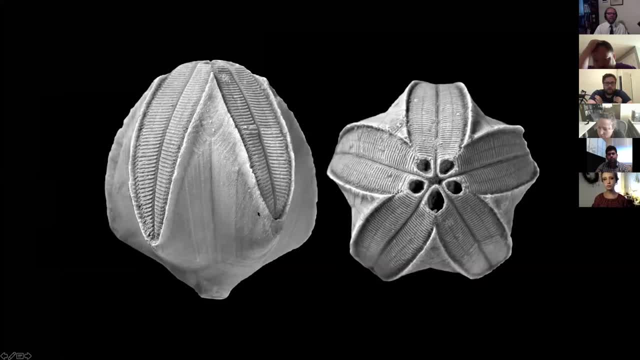 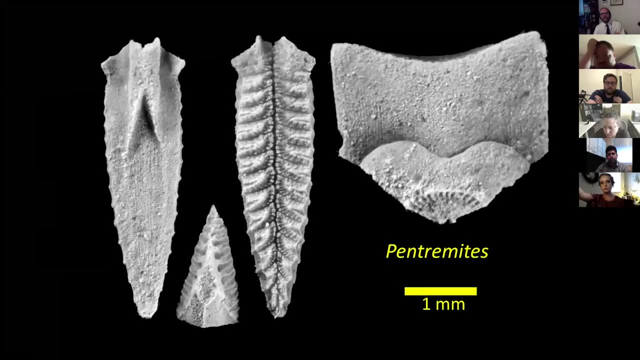 It's not so much a taxon as much as an age category. This is the most common blastoid there, the Pentromytes, and you see the beautiful preservation at this locality. But based on the morphologies you can see here, you can identify. 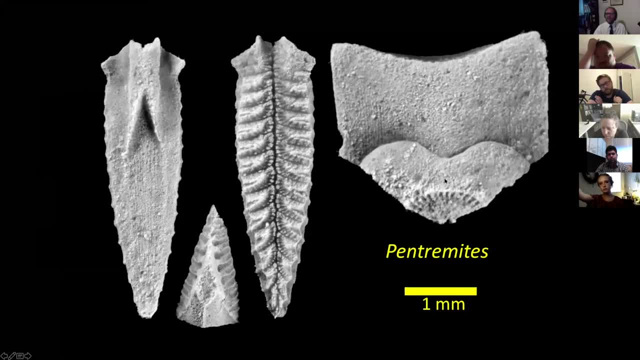 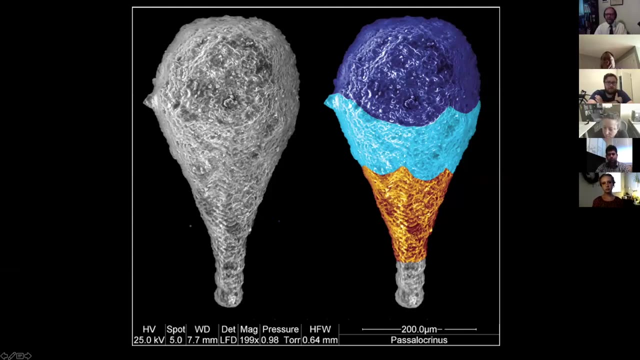 Okay, You can identify all the different parts of the blastoid from the sediment. This is a basal plate. these are lancet plates, deltoid plate- okay, Pretty straightforward stuff. This is a Pasilocrinus. You can see the scale on this. that's 200 microns. 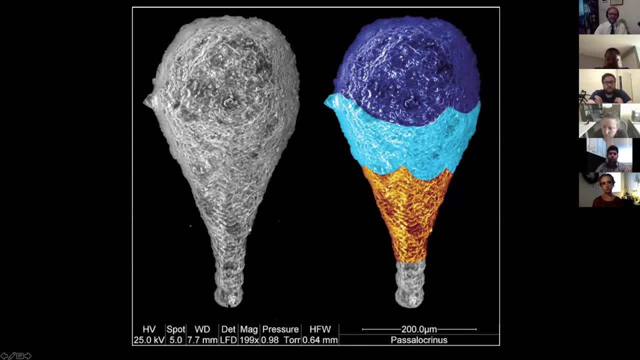 That's the top of the blastoid and there's three stem columnals coming down off the bottom of it. This is actually the most common echinoderm at the entire locality, Believe it or not. I had a student do undergraduate research and from a couple of samples weighed 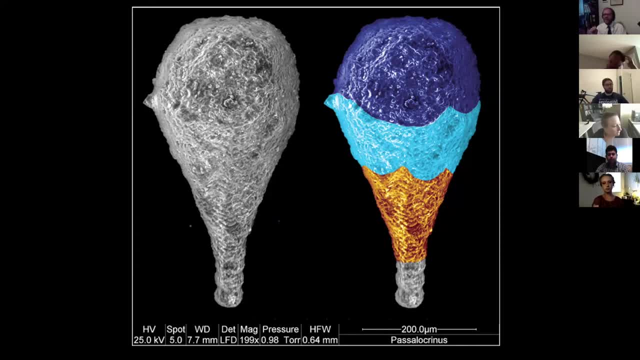 and washed calculated 37,000 of these per kilogram of sediment, So these are amazingly abundant. But again, 37,000 things that are 200 microns high isn't actually all that much material. So we have a lot of sea urchins. 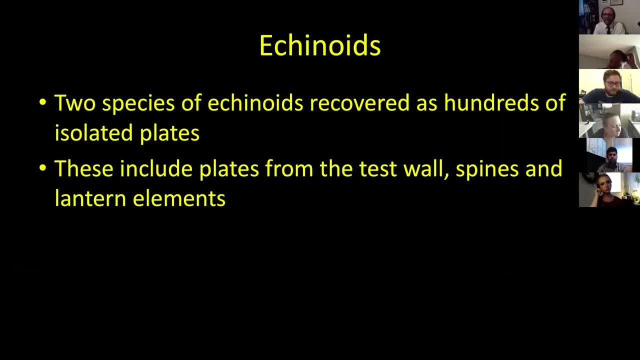 Sea urchins. We didn't see any sea urchins at the locality, but we have lots of sea urchin parts. We have them from all over: the animal: the tests, the spines, the lantern elements. They're all there in the sediment if we know what we're looking for. 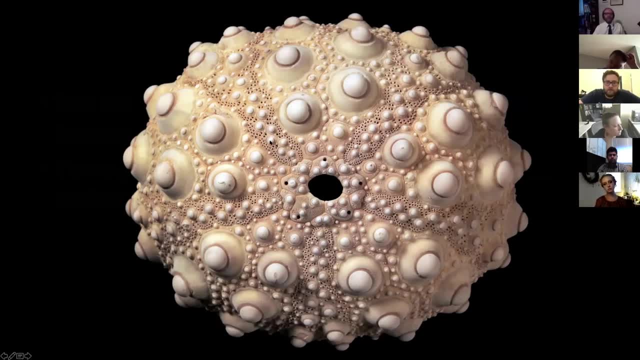 So that's a modern sea urchin You can see on the outside. we have some of these pieces with two holes. Then we have these ones with the big knobs on them. These are where the spines attach, And then here's material from the sediment. 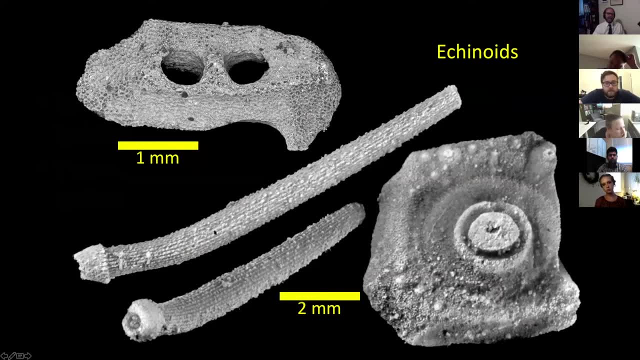 Here's one of the plates with two holes in it, Here's a spine And there's one of the ones with the knobs on it, So we have the whole animal from the outside. This is the inside of a sea urchin. 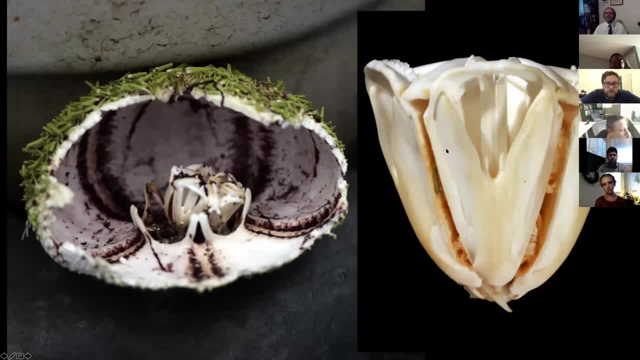 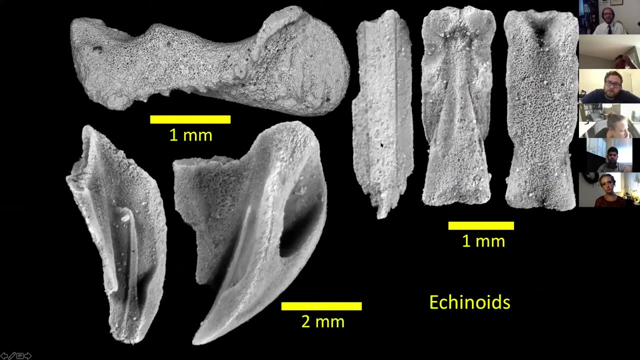 That's the lantern, That's the mouth apparatus And you can see it has a big tooth. here. This is called a pyramid And it has this called a rotula over here and some other elements And in the sediment we have these. 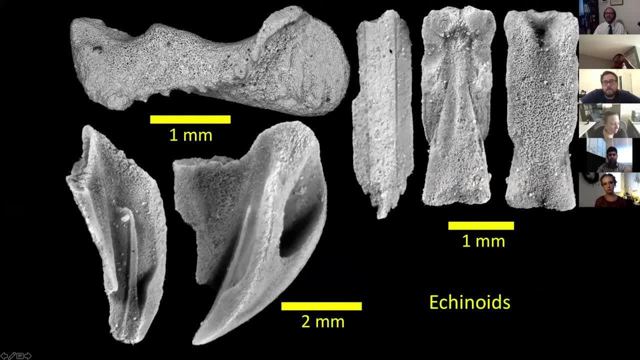 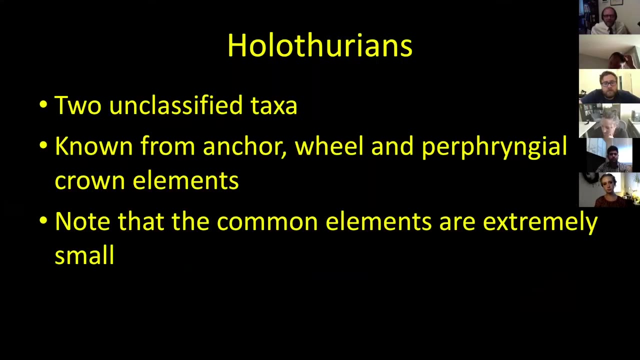 That's the pyramid, That's the rotula, That's the tooth, That's one of the upper elements on the lantern. So all the parts are there, But you wouldn't recognize them unless you knew what you were looking for. Holothurians are sea cucumbers. 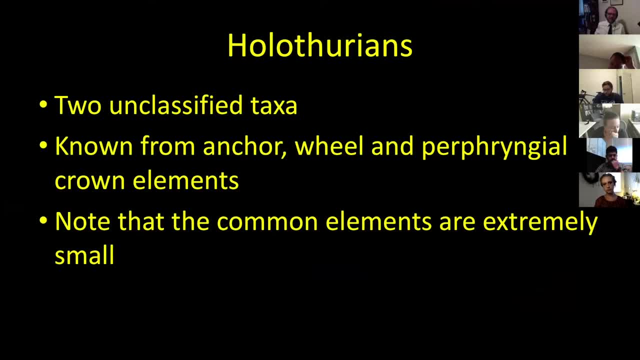 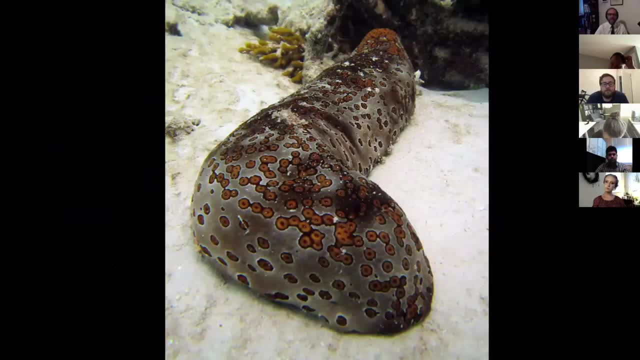 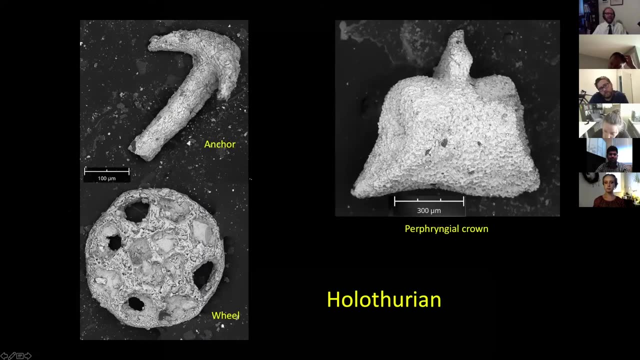 Sea cucumbers are echinoderms And they have. They have a huge number of skeletal elements embedded in their body wall, But they're exceedingly tiny. That's a modern sea cucumber. Doesn't kind of look like a crinoid very much. 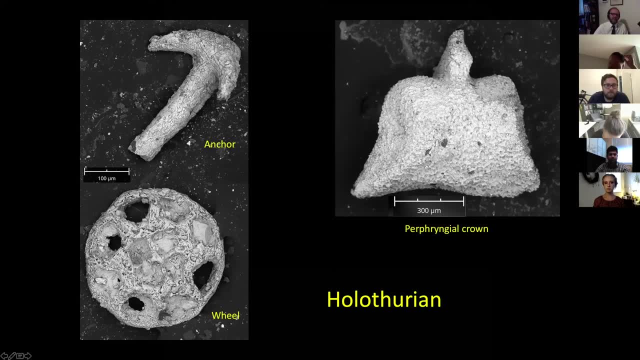 But these are sea cucumber parts. This is a wheel element, This is an anchor element And this is one of the ten plates around the throat of the animal. Again, you see the scale on these things. These are very, very small. 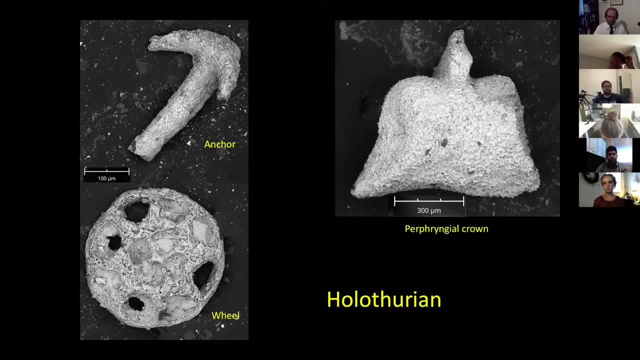 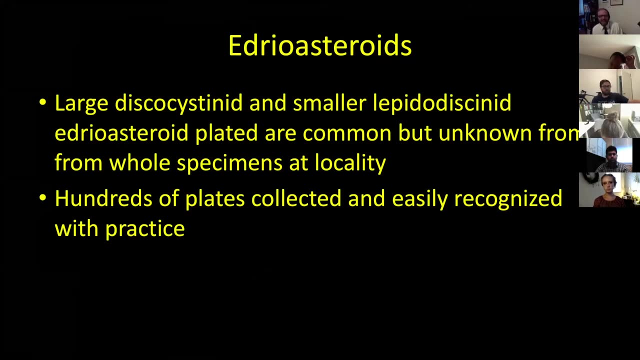 But they're in the sediment, Along with the animal, Along with everything else. If you know what you're looking for, I cut my teeth on edrioasteroids. Edrioasteroids are the first organisms I worked on, trying to straighten out what the individual 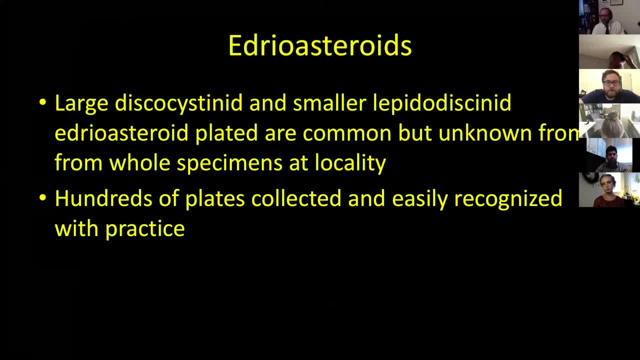 elements look like. While we have no edrioasteroid specimens from this locality, we have hundreds and hundreds of plates, And they're very easy to recognize once you know what they look like. These are whole specimens of the two types we have. 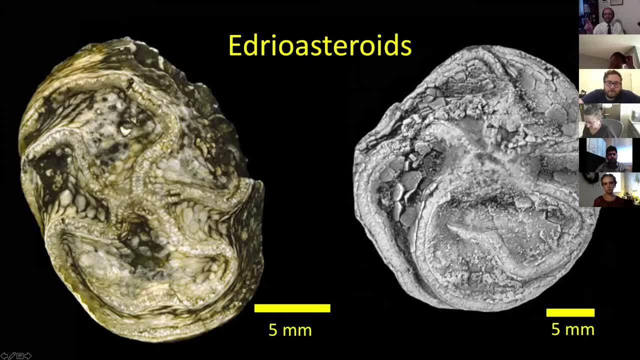 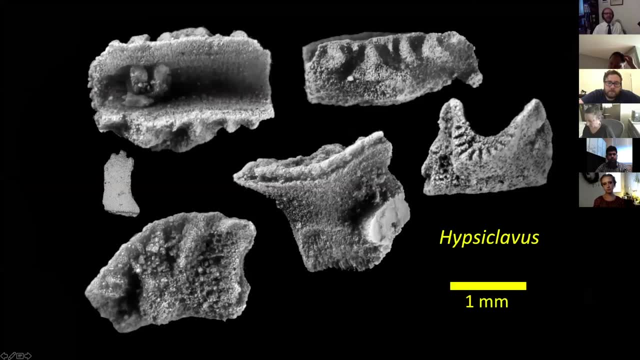 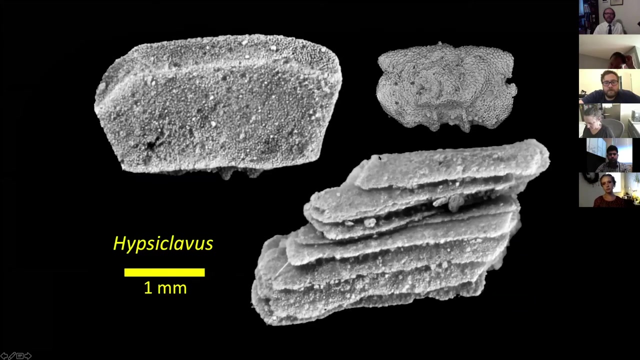 This is called a discocysteinid- Yeah, Disco. And this is a lepidodiskinid. These are some of the plates from the arms. These are what moves the food along, That covers it. This is the edge of the mouth frame. 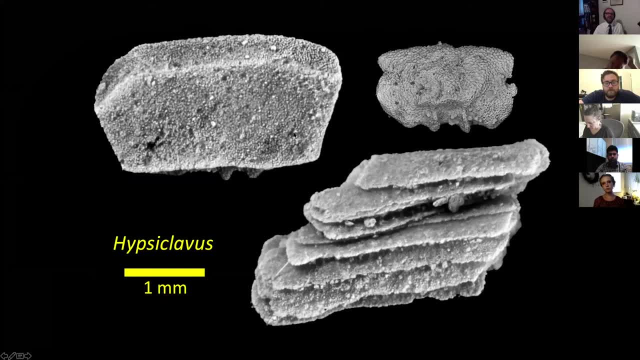 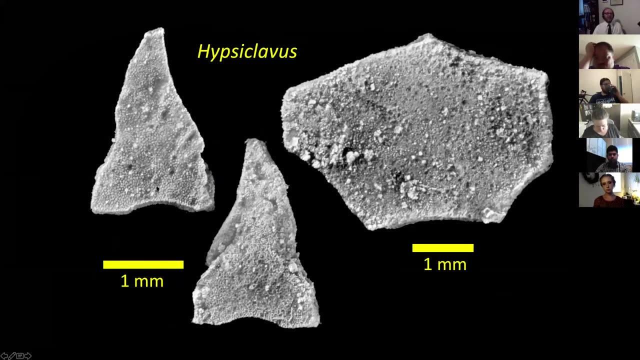 These are plates from the bottom of the animal. This is what's called a recumbent zone plate. That's part of the holdfast And this is the flexible stock, The plating of the body wall, And this is the plates that cover the anal opening. 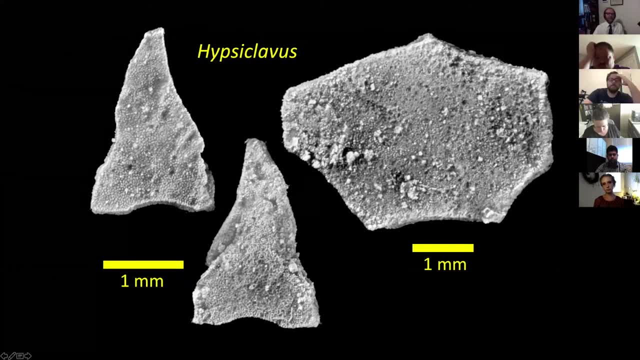 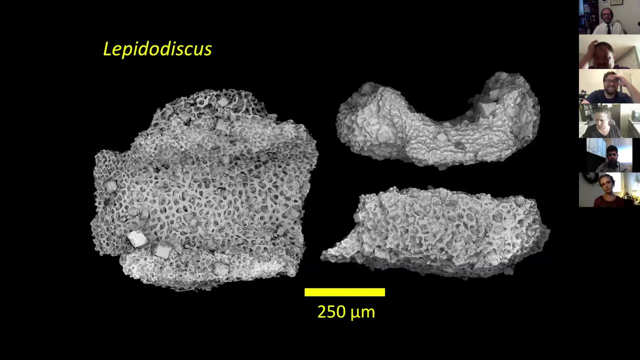 Not many on these on an animal. And there you go. You've now seen an anal plate of an edrioasteroid. Your life is complete. The other species? I only know it from a few elements of the animal Arms. I know what this is and I know it doesn't look like much to you. 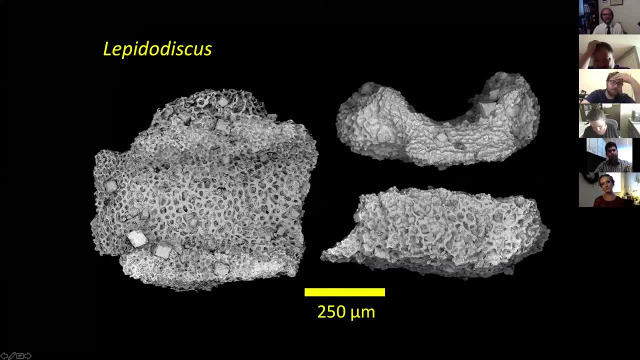 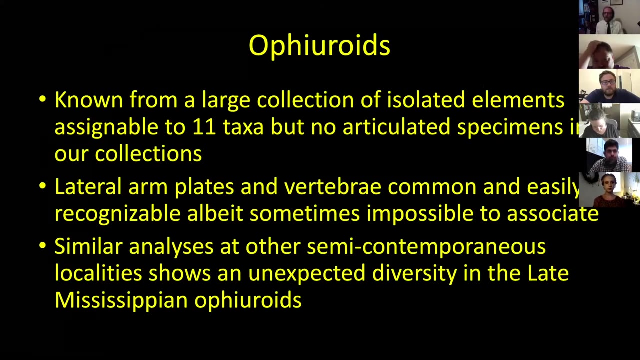 There's really nice dolomite here. But based on this imbricated edge here I can tell you it's lepidodiscus, So I can identify this one down to the genus pretty easily. So those kind of those organisms all had fairly, I would say, not unusual levels of. 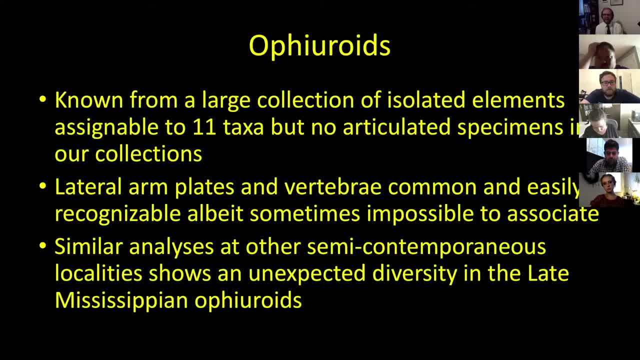 diversity. What I didn't expect when we started this project- and in fact, when you go to Nick Smith's defense on Wednesday, you'll see a lot more of this from another locality where Nick is working is you'll see that the brittle stars, the ophiroids, have a diversity that 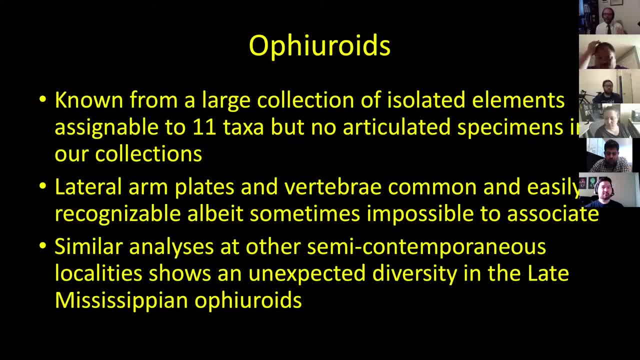 is unmatched in the Paleozoic, But we only know about it from these disarticulated elements. At this particular locality we have 11 taxa, But we don't have any articulated specimens. The lateral armplates and the vertebrae are ubiquitous in this material. 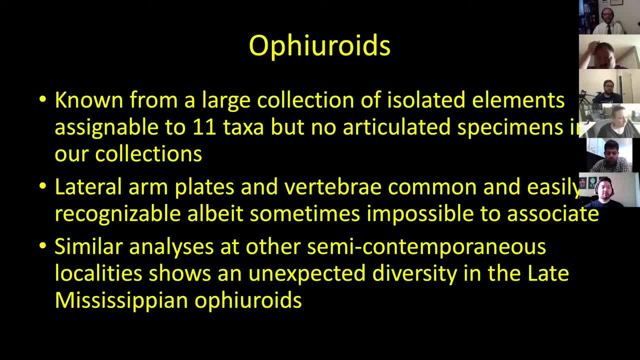 They're very easy to identify once you know what they look like And, very importantly, if you look at semi-contemporaneous localities, which we have, this, what we're seeing in this locality, is not abnormal. This is typical. Nick has the same level of diversity in the Sulphur indium. 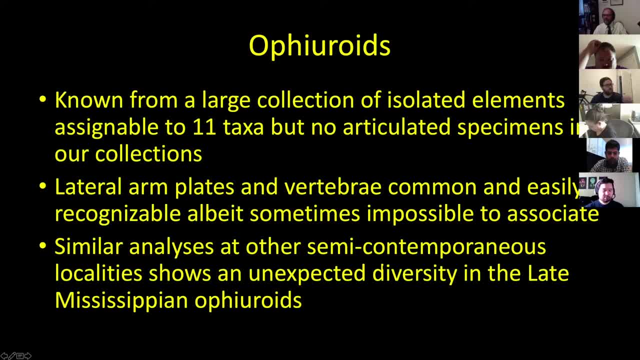 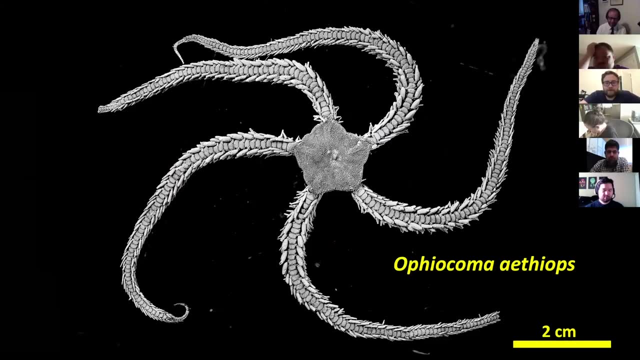 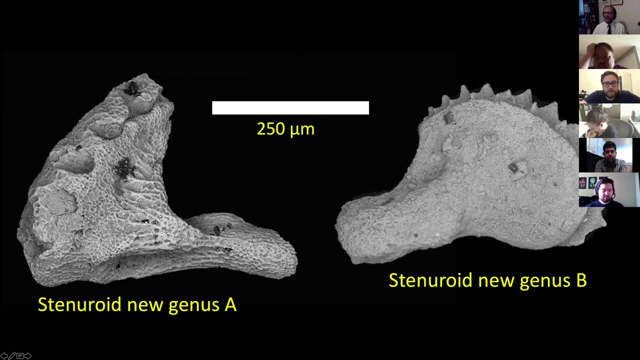 a local sulfur indiana locality. we have nearly the same diversity in a in a uh locality right outside of st louis. that's about the same age, so this is normal diversity for this and that would be a brittle star. we have a couple of different species at this locality of things called stenuroids. 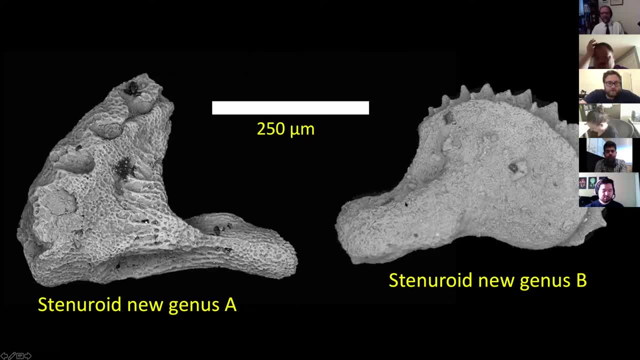 stenuroids, lateral arm plates sort of look like uh rackets with a peg on the end. i and these are the little facets for the uh, for the spines coming off. interestingly enough, this is upper mississippian. the youngest known stenuroids in the literature right now are in the devonian, so this extends. 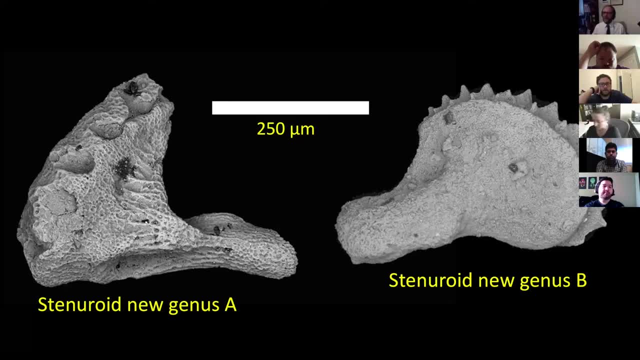 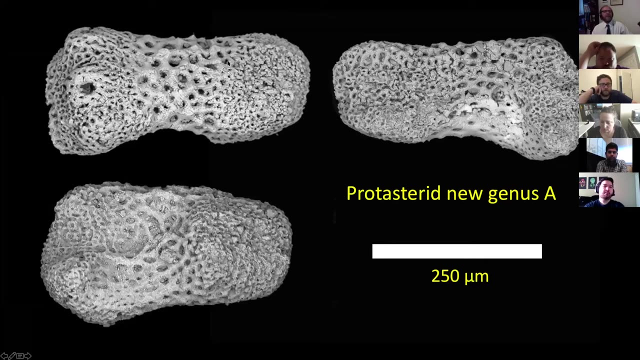 these from the end of the devonian all the way through the end of the mississippian and we have diversity. this is the most common brittle star at this locality. it's this group. we have a protasterid which is kind of a weird looking thing with this. 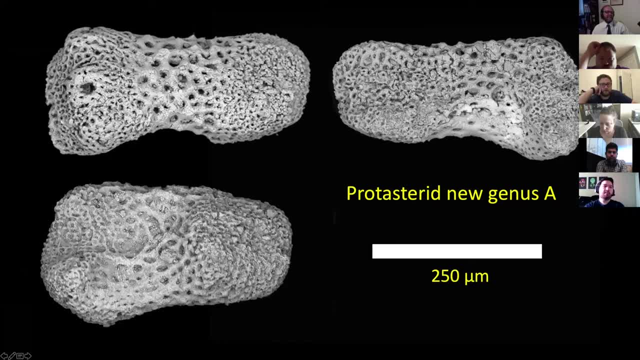 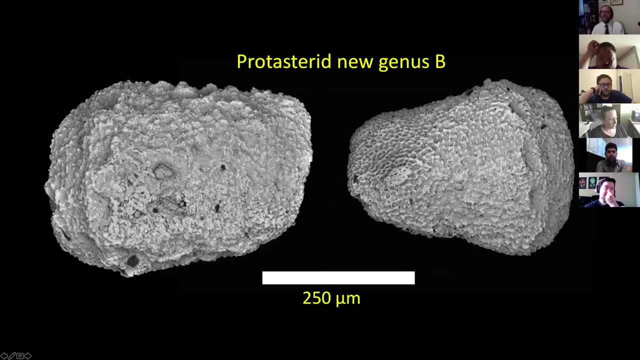 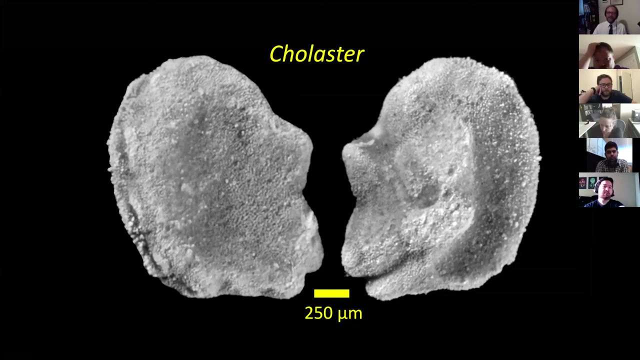 big stereome here and these are the spine facets. another protasterid which varies clinically and where the spines attach, and some details here and there, but it's a different one. we have a thing called cloaster. this one's the big one, so you can see that these plates here. 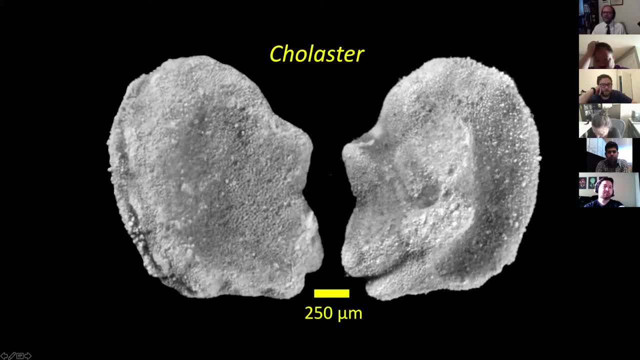 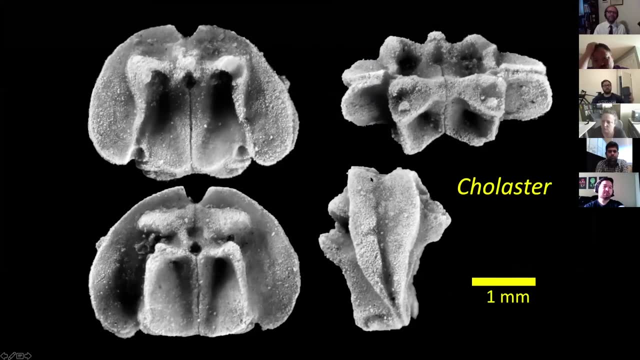 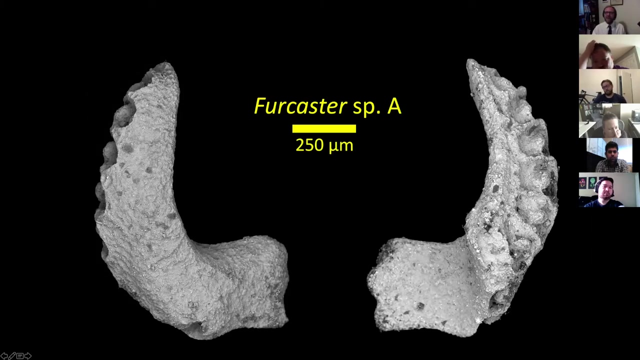 are pushing two millimeters across. so these are. this is the only brittle star where the plates are over a half a millimeter across. these are the vertebrae of the same. we have two species of furcastrid. this is a sort of a sickle shaped guy here. we call it species a because why not? 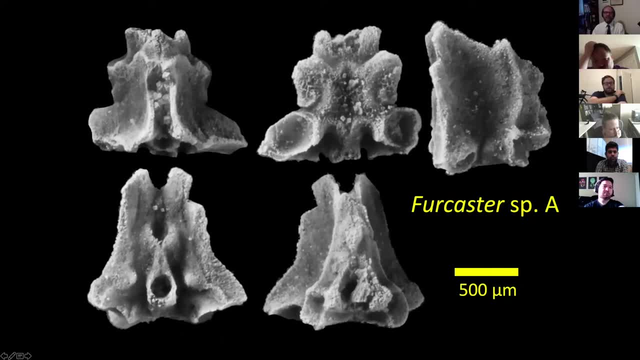 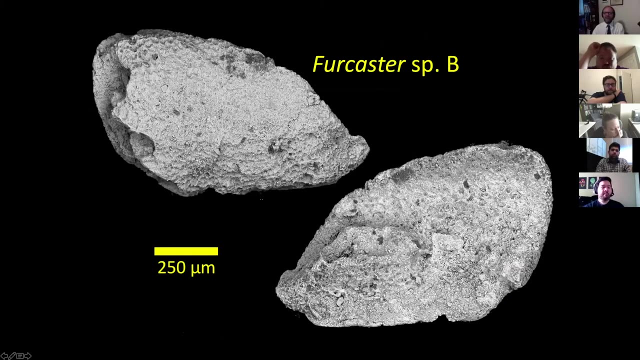 we have the vertebrae that we can associate with this, based on a couple specimens that that were given to us by by a collector in alabama. this is the other furcastrid we have here. it's a lot longer plate. it's not so sickle shaped. 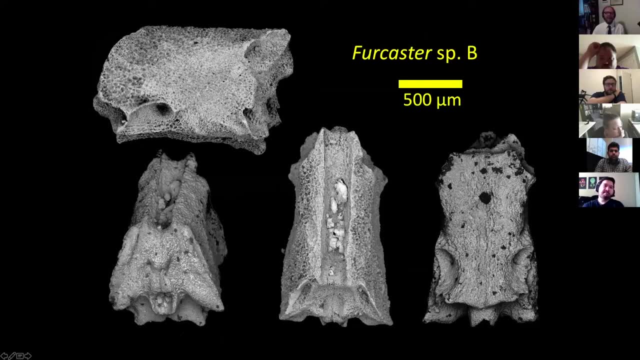 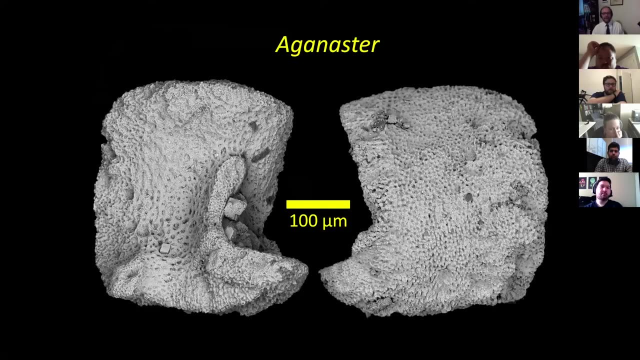 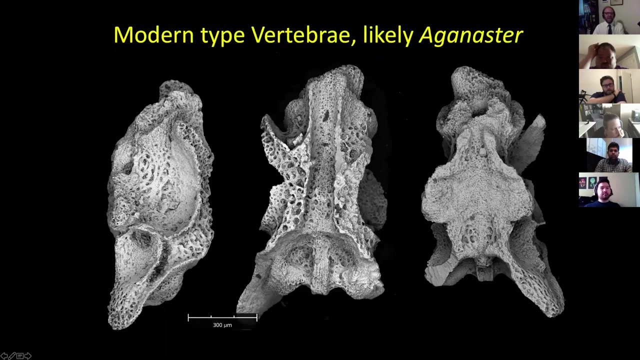 the associated vertebrae. here again, with that really nice preservation, We have an agonaster. An agonaster belongs to the modern group of brittle stars And the vertebrae associated with that appear to be this thing which, frankly, I think looks a lot like a giraffe skull, but that might just be me. 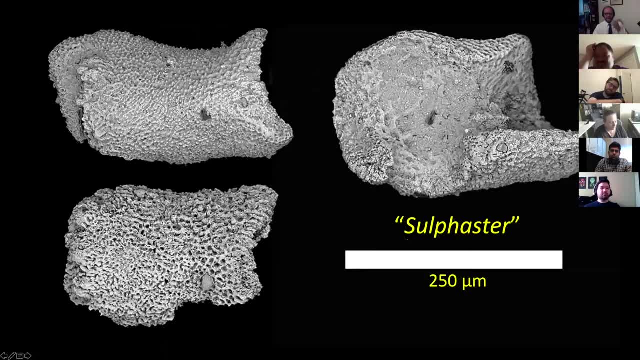 We have this new thing that Nick's naming, called Sulfaster, named after Sulphur Indiana, And again, this one's exceedingly small. This is just a quarter millimeter long, And we have a couple things that we really we know. they're brittle stars based on their 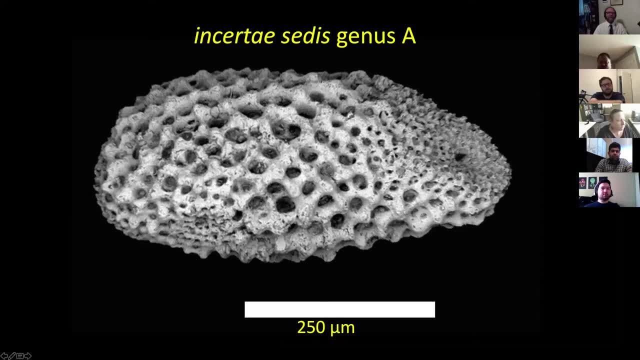 morphology, but they're really defying our ability to classify them. So we have a couple of things that we really we know they're brittle stars based on their morphology, but they're really defying our ability to classify them. So we have a couple things that we really we know they're brittle stars based on their morphology, but they're really defying our ability to classify them. 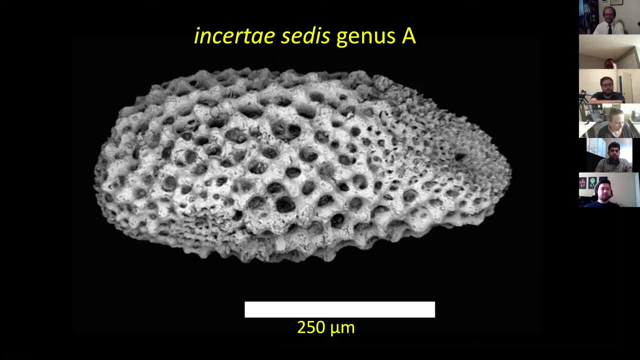 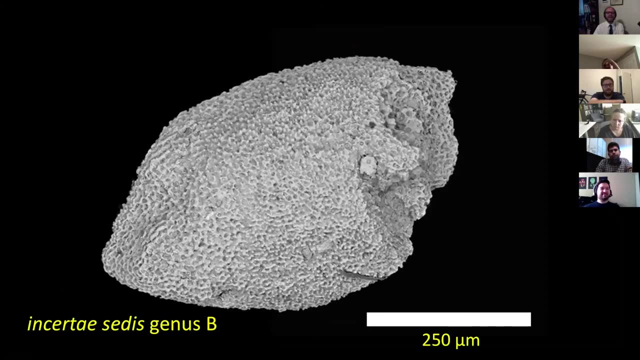 right now. This is, we just put it in- insert a. see this, which is Latin, for I don't know what it is, But it's a different kind of brittle star that we haven't seen. This is another weird one, has these two great big facets on the front, and we're 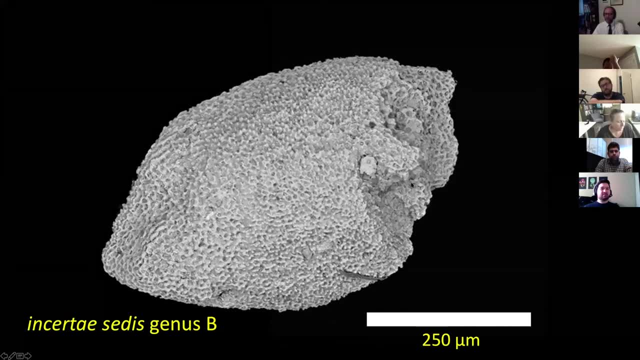 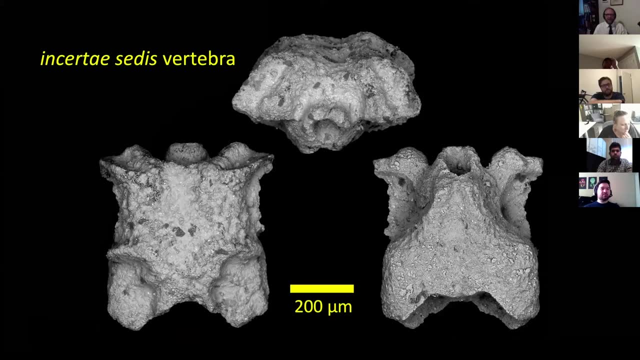 not really sure what this attaches to, but it is different from the other ones that we've seen, And it's often very difficult to place the vertebrae. And it's often very difficult to place the vertebrae with the lateral arm plates. 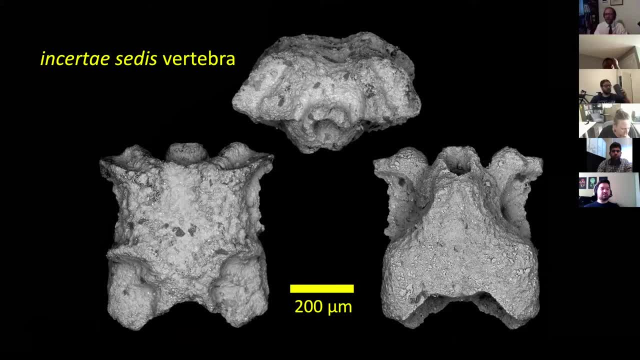 So we have a lot of vertebrae that we don't know what they belong to. You can identify the taxonomy is based on the lateral arm plates, So we just have these. we call this one the pluck chicken. looks like a roasted chicken. 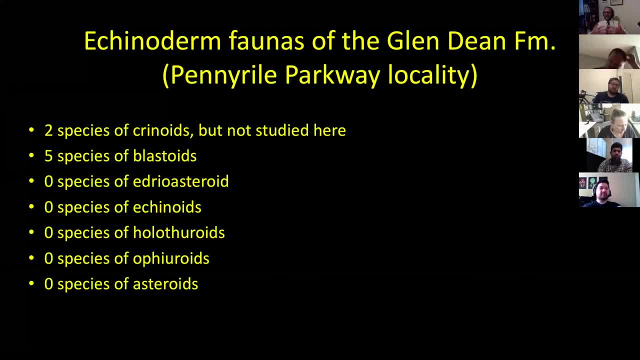 So what we see, then- I think I hopefully have shown you- is that there's a fundamental difference. So what we see, then- I think I hopefully have shown you- is that there's a fundamental difference in the level of debris. in the level of debris, 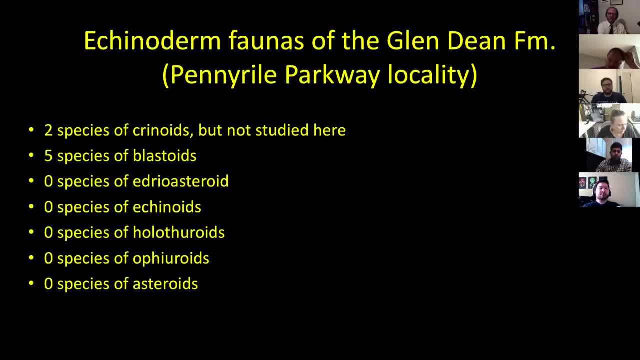 We see at this locality, depending on the methods we use. If we go back to our original 30 man hours crawling over the outcrop level of trying to see what the echinoderm diversity is, We had two species of crinoids. 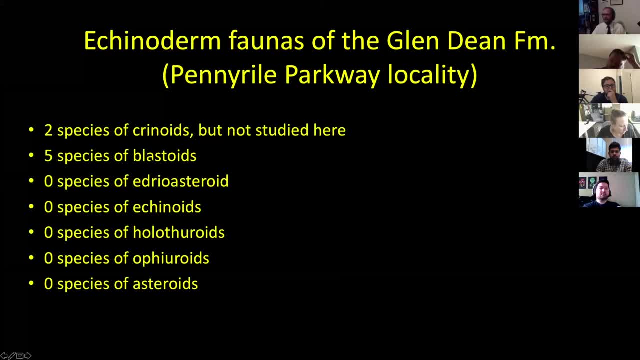 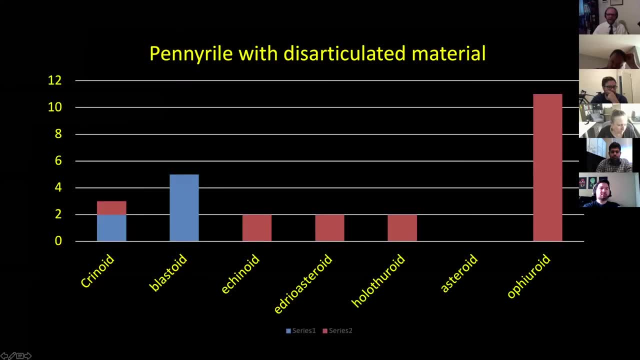 We have five species of blastoids and nothing else at this world famous fossil locality. We have five species of blastoids and nothing else at this world famous fossil locality. This is what we see: We have five species of blastoids and nothing else at this world famous fossil locality. 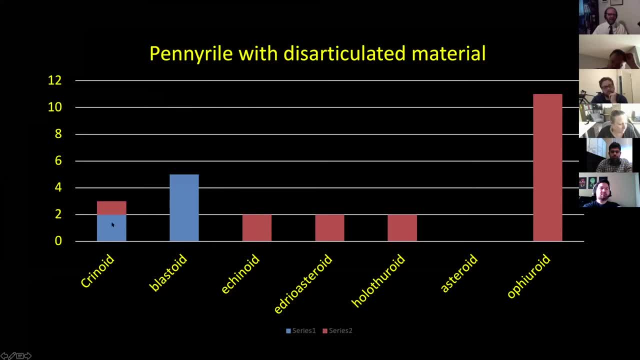 We have five species of blastoids and nothing else at this world famous fossil locality. If we add in what we know from isolated elements- ignore what the crinoids are- the crinoids would probably be way off the graph here, but I don't have the skill set to understand that crinoid data. 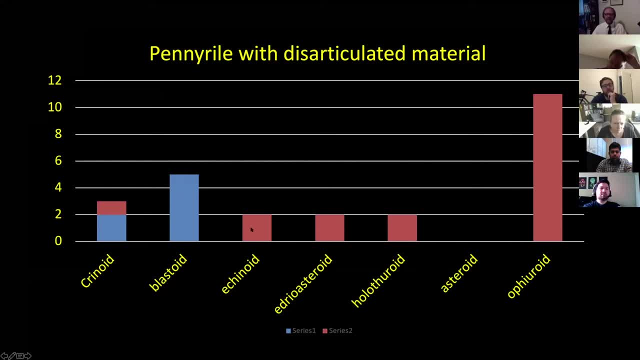 But I don't have the skill set to understand that crinoid data. The blastoids didn't change, but we added echinoids, two species, edrio asteroids, two species, sea cucumbers, two species and 11 species of brittle stars. 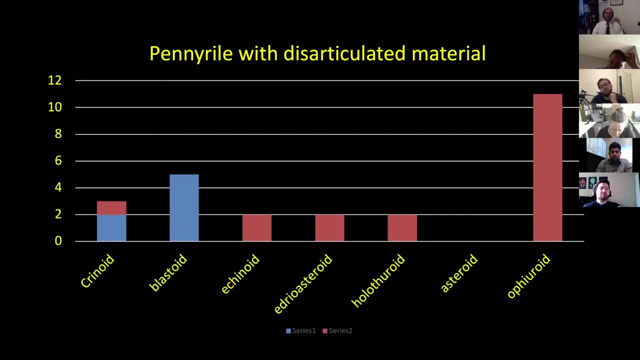 That's fundamentally different. That's fundamentally different. So, at least at a very initial level, we can say that, yes, if you only sample haphazardly on the surface, you will get a diversity pattern that is muted with respect to what is actually there. 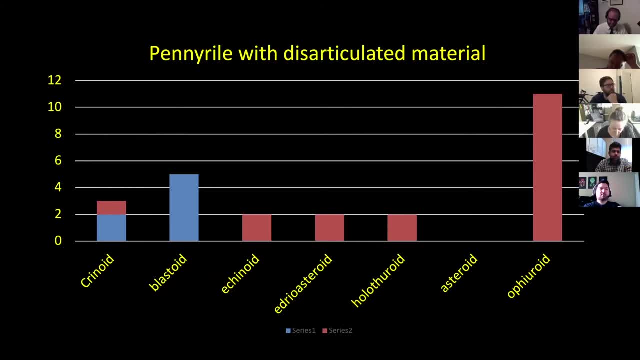 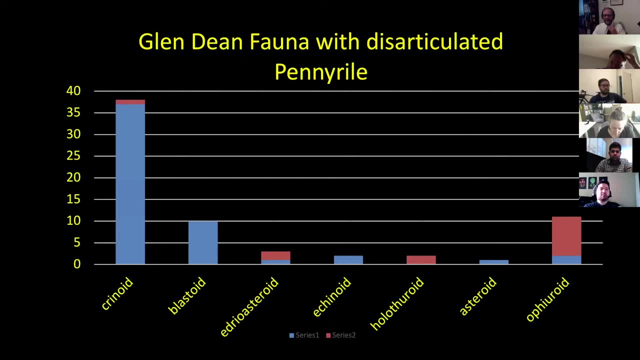 if you look and you know what you're looking at, if you look and you know what you're looking at. But can this change the global pattern? Well, I think it can, for Well, I think it can for well, I think it can, for here's the fauna from the Glendene. 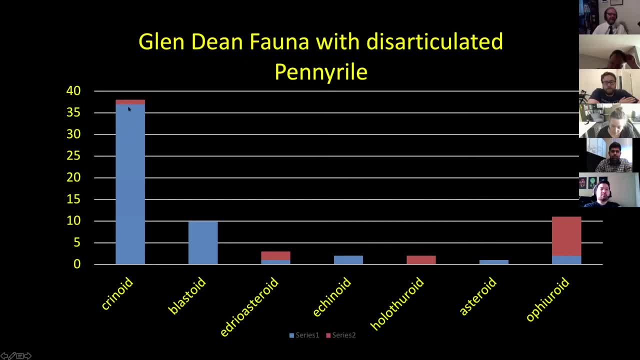 here's the fauna from the Glendene. Over here we had 37 species of crinoids described by Ettingen and Chestnut. Over here we had 37 species of crinoids described by Ettingen and Chestnut. 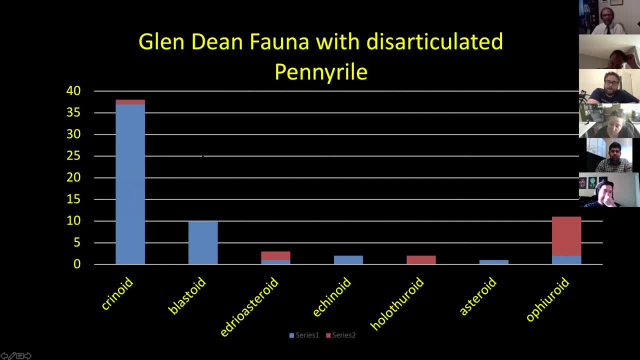 We added one. We probably could add more if I knew anything about crinoids Blastoid fauna. we haven't really changed it that much. We added two new edrio asteroids to the fauna. We already had the two echinoids. 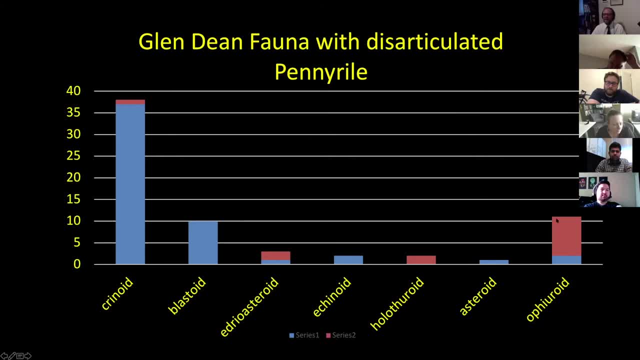 We added two sea cucumbers and nine species of brittle stars to the fauna. We added two sea cucumbers and nine species of brittle stars to the fauna, So this formation's diversity has skyrocketed. in terms of the ophiroids, which went from relative obscurity to the second most abundant group of echinoderms, 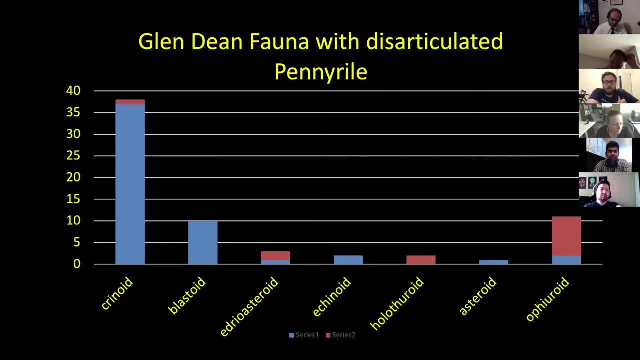 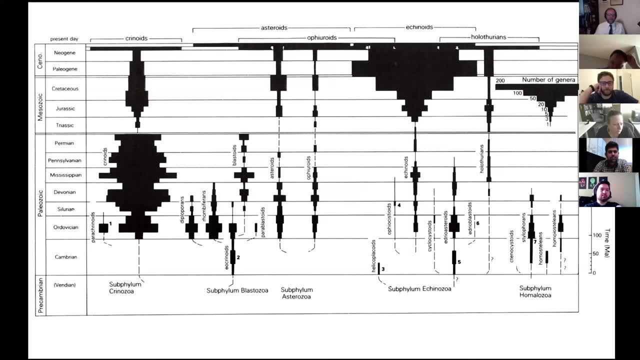 because we looked at it in a different way. And then, if you bump this up even further, this is the famous echinoderm compilation of diversity from Sprinkle And these spindle diagrams are: just think of these as bars. And these spindle diagrams are: just think of these as bars. 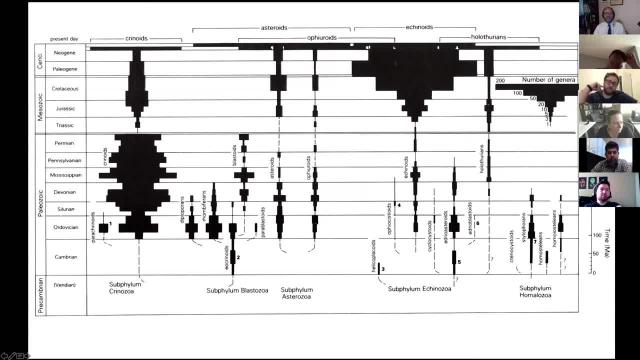 So this shows you the relative amount of diversity at different times through Earth's history by the width of the bar And the pattern of ophiroids is actually very interesting. It's really low-level diversity throughout the Paleozoic until you get to the end of the Mississippian. 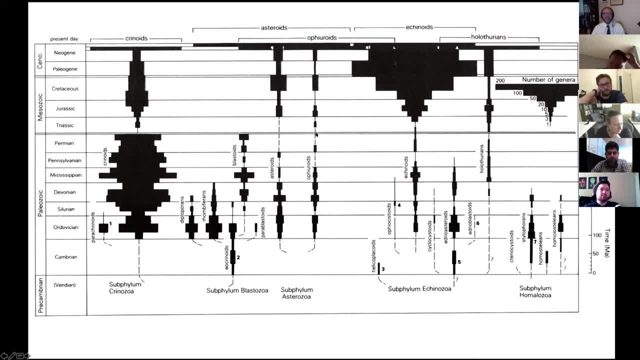 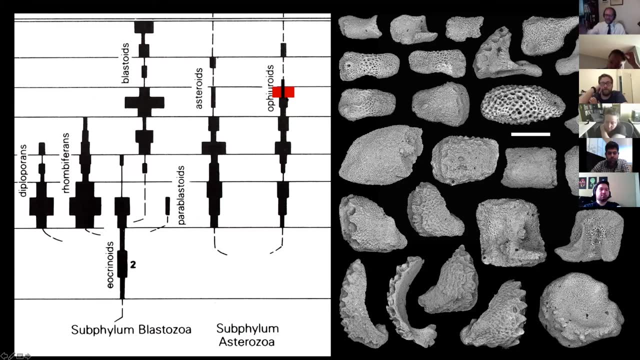 And then it's basically nothing. there's a couple taxa here until you get well into the Triassic. What happens? when we look at it, The highest level of diversity in the Paleozoic is that one locality. There's more diversity in the Paleozoic than any other time in the Paleozoic. 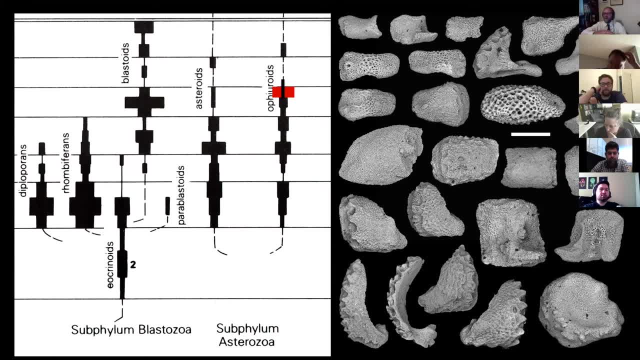 when you sum up every brittle star that's been described everywhere in the world. It's staggering the changes you see here. And then you put it up with again, the diagrams like this: these are the plates that are going to the proposal I'm working on. 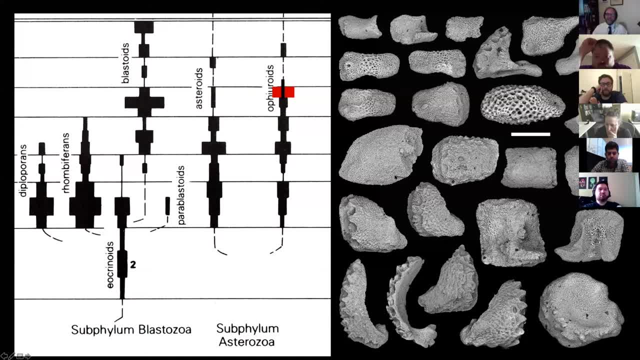 of just all the different types of diversity here, And then, if that weren't enough, Nick has 11 species in his locality, and those 11 species include three I don't have, And they're the same age. So really, this bar is even wider if we put all the data in. 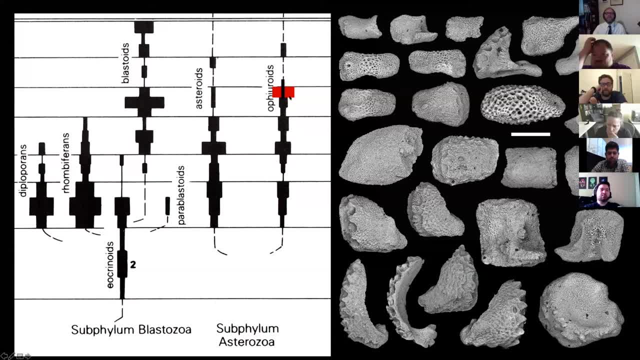 So what we're going to do from here on out is we're going to try to duplicate this throughout this section and see what the real diversity is in brittle stars through time And what's going to happen based on a few initial samplings that we've done. 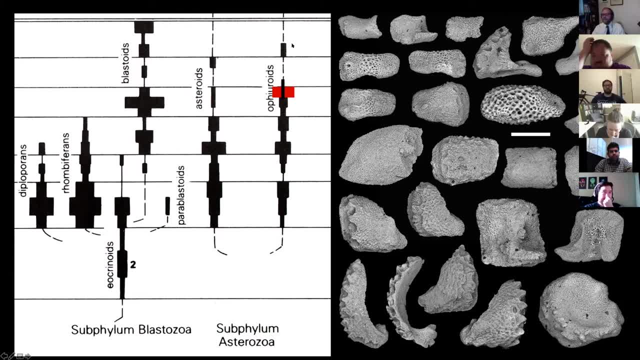 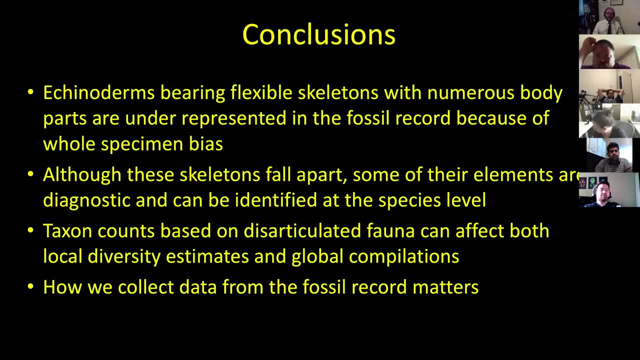 is. it's all going to look like this all up here. So we're fundamentally rewriting the diversity of a group through time because we're using a different methodology. So, in conclusion, echinoderms that have very flexible skeletons with huge numbers of body. 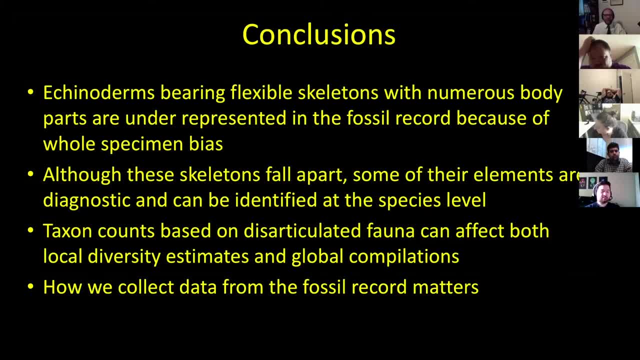 parts are going to always be underrepresented in the fossil record because there's a specimen bias, where we study specimens that are complete rather than studying specimens that have disintegrated. Although these skeletons can fall apart, some of the elements are going to be separated. 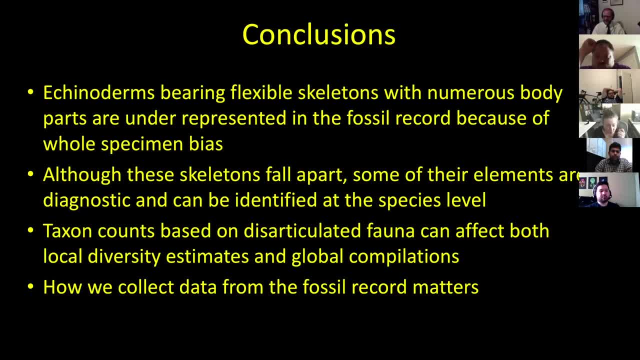 And that's going to be a big problem. So echinoderms are diagnostic and can be identified at the species level. Taxon counts based on disarticulated faunal elements can affect local diversity and the estimates for global diversity. compilations. 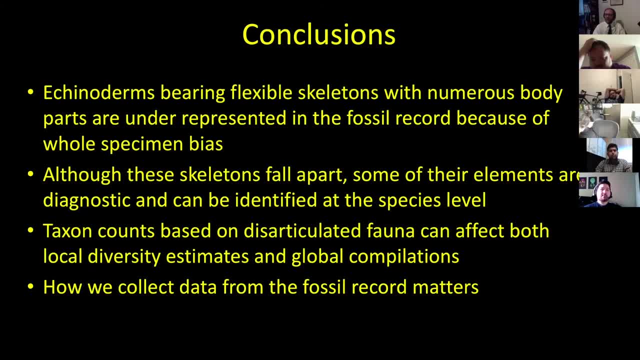 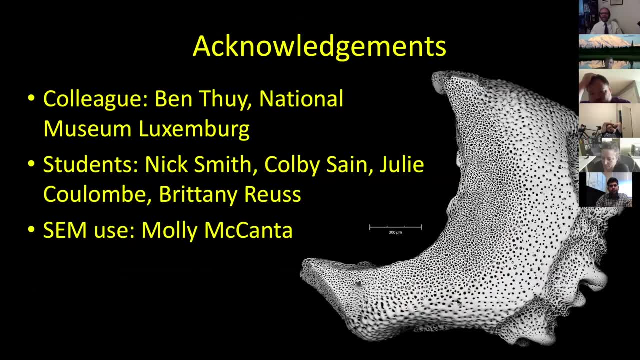 In other words, how we collect data from the fossil record really does matter. Okay, Oop, And I'll leave it there And I'll entertain questions for a while, So I'm going to go ahead and start the show now. 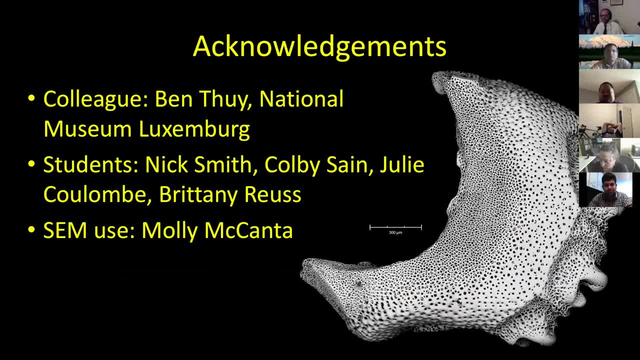 And then I'll let you know if you want to speak about that. Okay, Okay, Thank you, Colin. Thank you, Colin. This is Steve Rominello. Hey, Hey, Hey, I have a question. Yep, Totally sold on this idea. 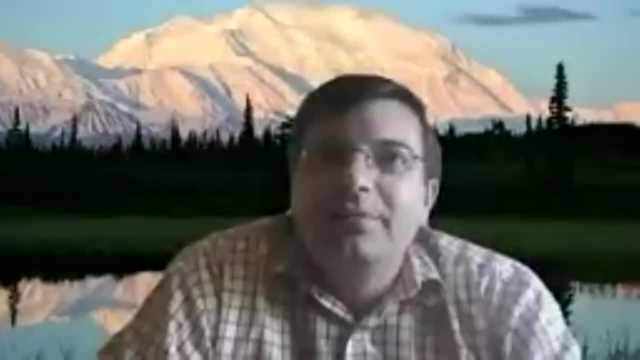 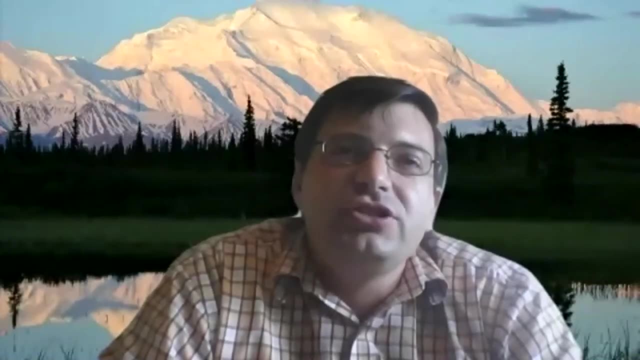 And I think this is awesome and I think you're totally right about it. But the question is how to implement it practically, right, Right, Because we've got so much rock to look at and it takes such specialty knowledge for each group of organism. 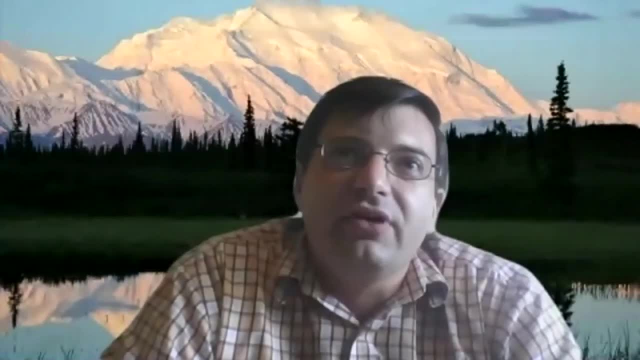 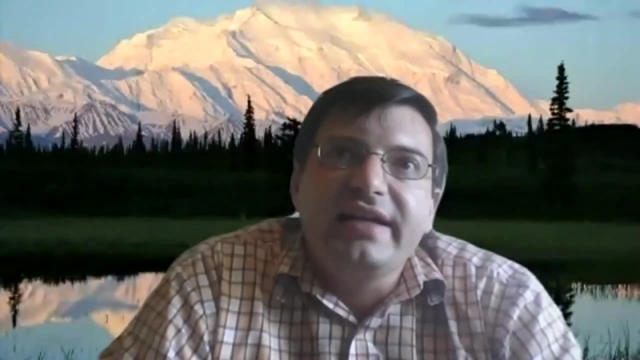 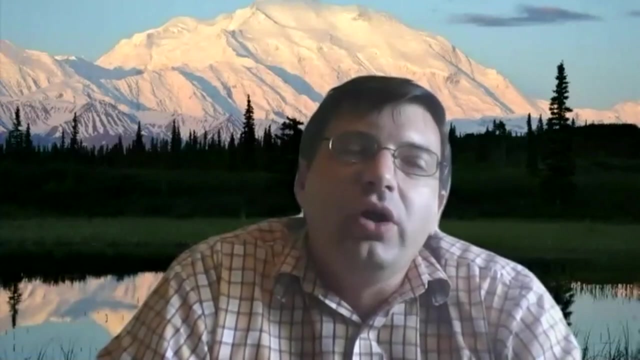 And you really have to do a lot of picking and separating Right. So I'm curious: do you think of efforts to use, you know, automated image classification systems, like the way that Google finds pictures of cats Right? Can we train You know? if there was a substantial effort, let's say I don't know how many million dollar effort. 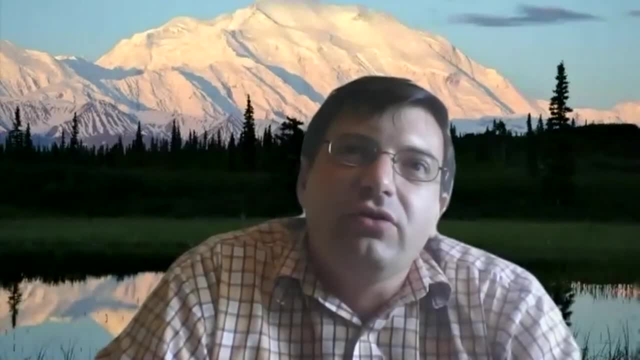 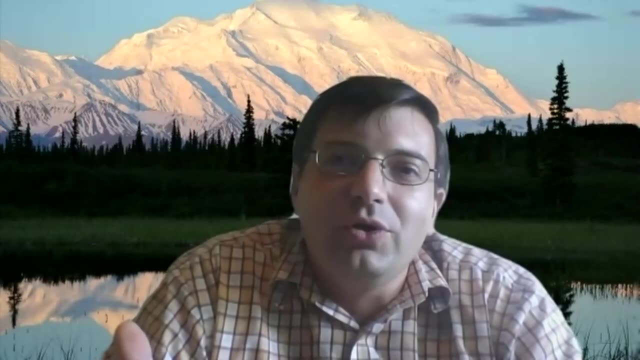 Could we train automated detection systems to look at these microfossils and begin to sort of, because a human will never be able to look at all of these. A human will never be able to aggregate everything we know about the fossil record now. 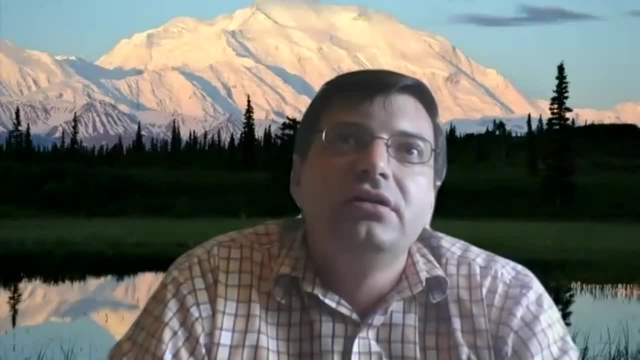 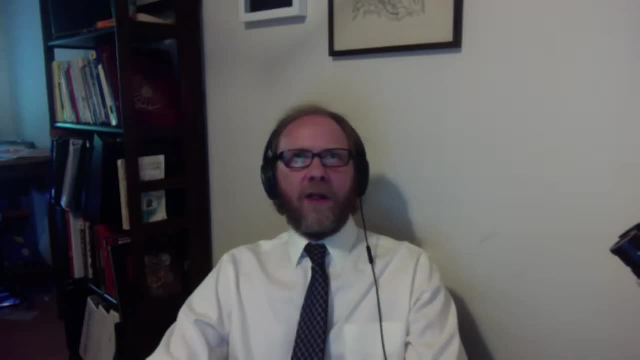 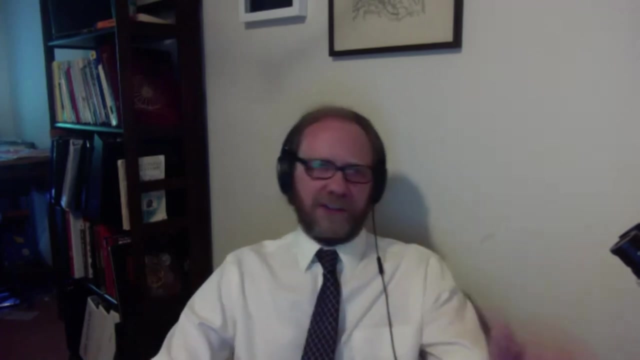 But a substantially scaled computer algorithm probably could. Right, I would say the answer is yes and no. Yes is Once we understand what we're seeing. Yes, But the way the Brittle Star portion of this project evolved- and you can talk to Nick about this- 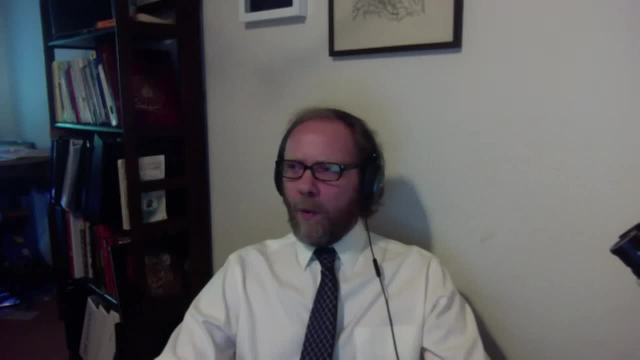 He was much more involved in the Brittle Star part was when Nick came in I said I've got this project, We're going to look at Brittle Stars, And he said: and I said there's only two problems. 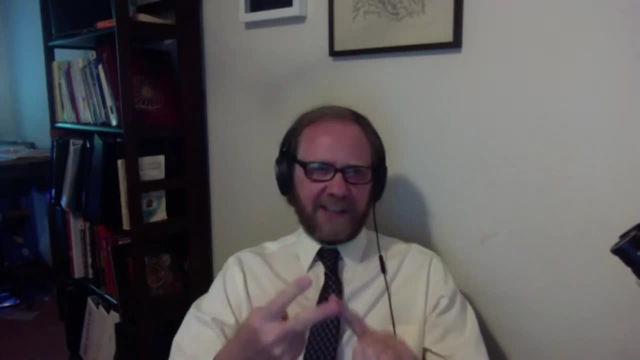 One is: no one has actually done any work on this, So we don't know what anything you're looking for Or actually looks like. And the second part was: I don't remember what it was like. Ask Nick, he'll remember it. 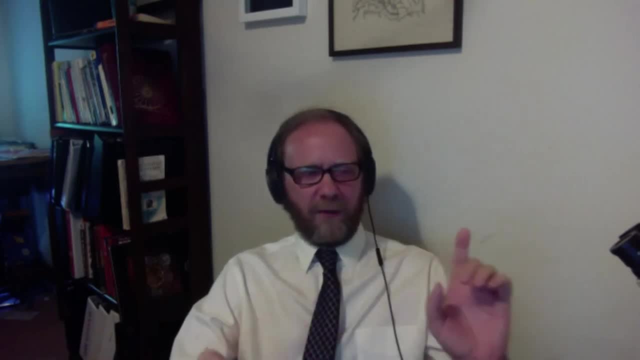 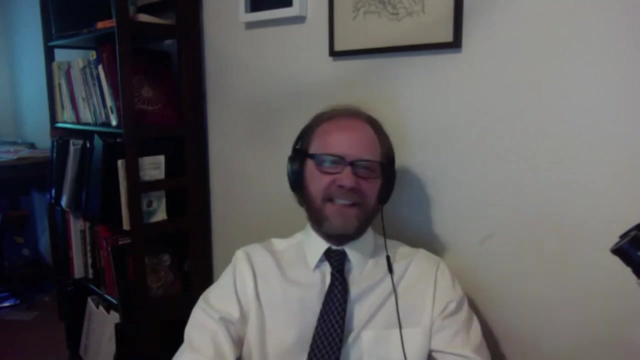 And when we started doing this, we were working with a colleague in Luxembourg who'd only worked in the Mesozoic, And so what kept happening? he said you'll know him when you see him. So we were just going back and forth between the SEM and emailing pictures. 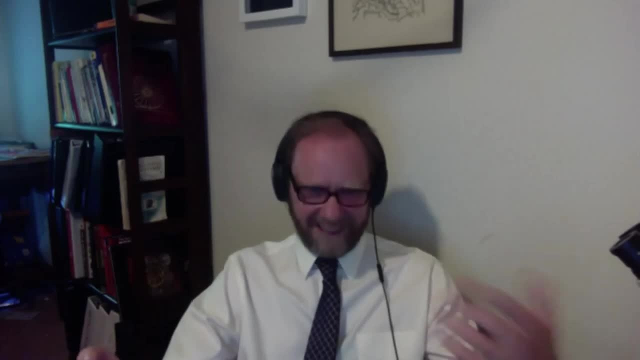 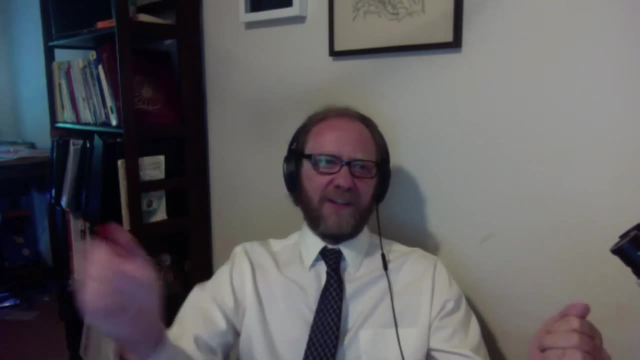 Saying: what's this? Is this one Yes? Is this one No? Is this one Yes? And we thought we had it all worked out. We had six or seven species. And then Nick went to Luxembourg and handed him some sediment. 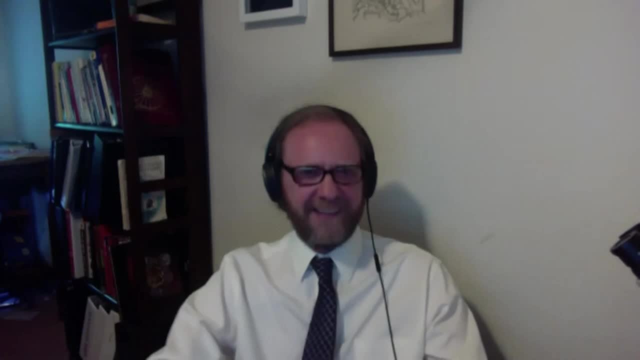 He put it on a train and said: well, you missed this one and this one, and this one and this one. So we are still trying to understand what these things look like. Once we know what they look like, they are distinctive. So when? 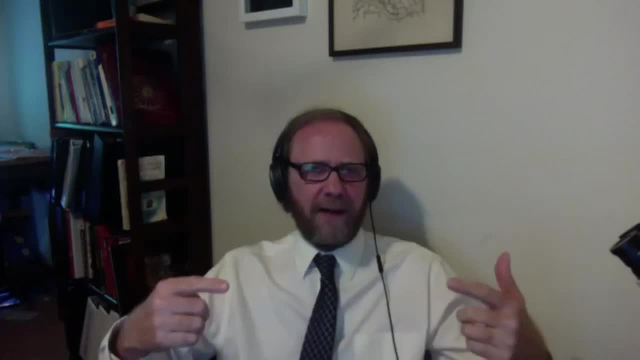 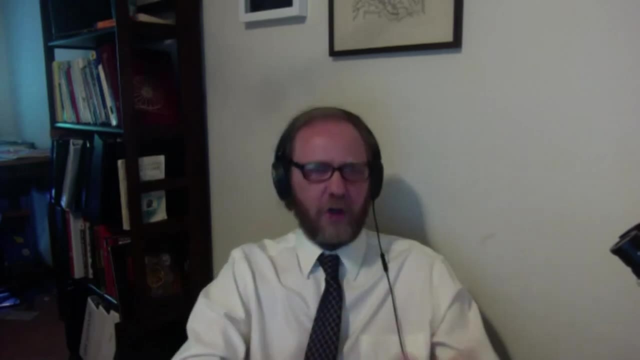 Every time we find a new type and we get it imprinted in our brains, we can see it, And from that aspect I think you're right. There could be a way to do that, But you can't do that until you actually know what they look like. 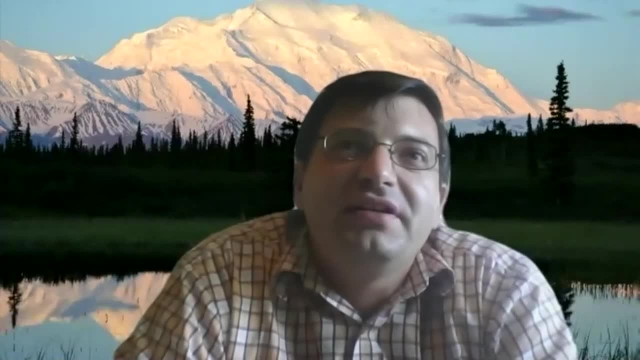 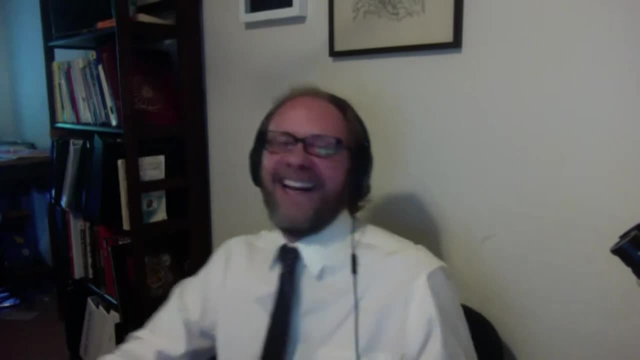 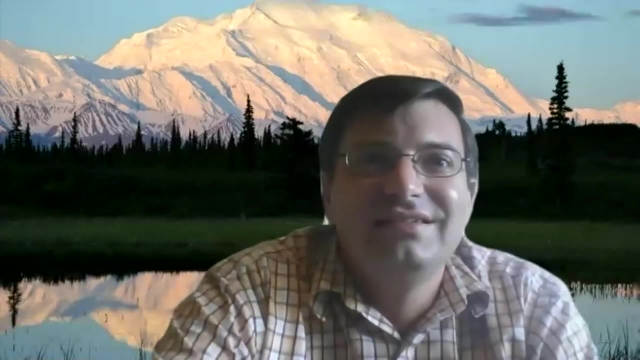 Yeah, I think the problem is that everybody's got a couple dozen of them imprinted in their brain And we need them all imprinted in one place. Well, everybody is- me and Nick, Yeah, yeah, yeah, Interesting. So a lot of what you were discussing was size bias. 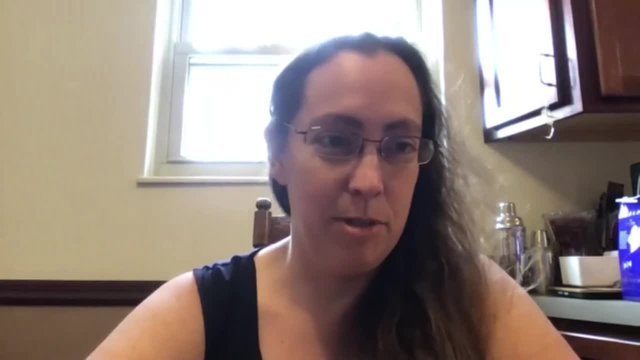 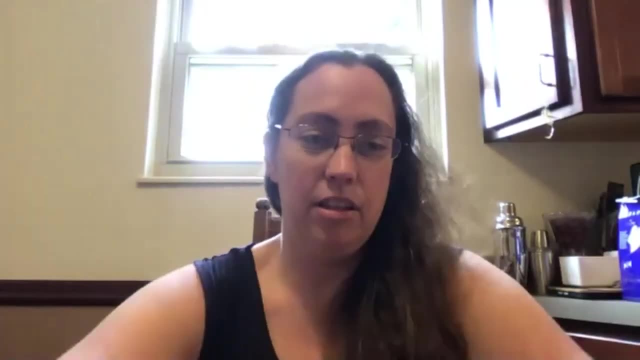 So what do you find when you're crawling on the outcrop versus what do you find when you actually are sieving it? Yep, Coming from my dinosaur project, how much of an issue do you have in a kind of paleo with basically trophy hunting collection? 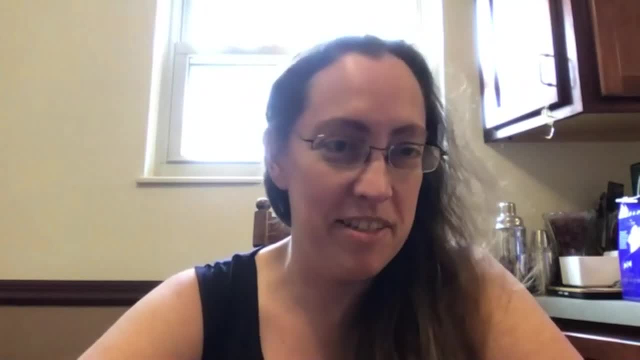 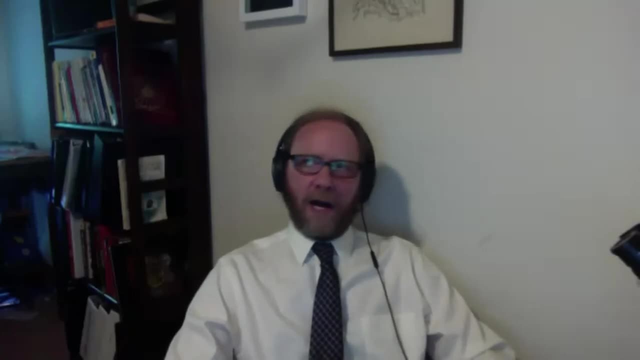 So only bringing back the most The most beautiful specimens and leaving behind even identifiable stuff in the field. That's huge Yeah. In echinoderms there's a big problem with trophy hunting for two reasons. One is trophy hunters take good stuff. 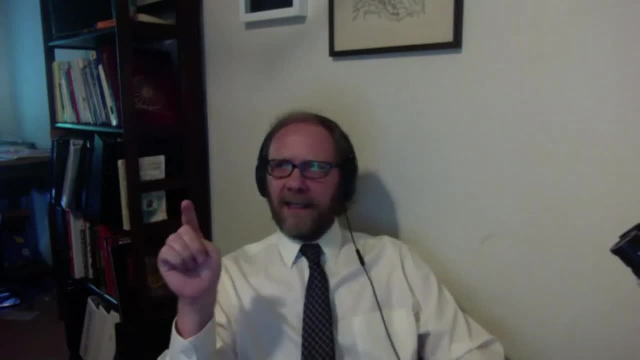 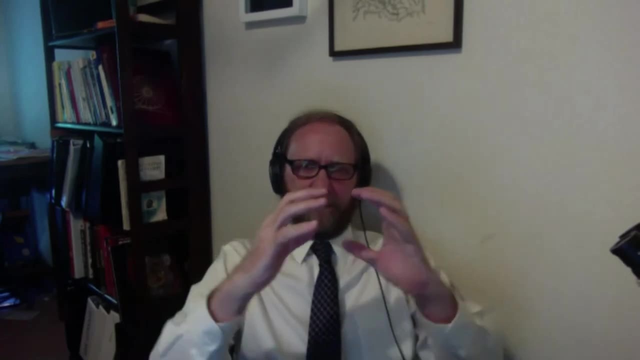 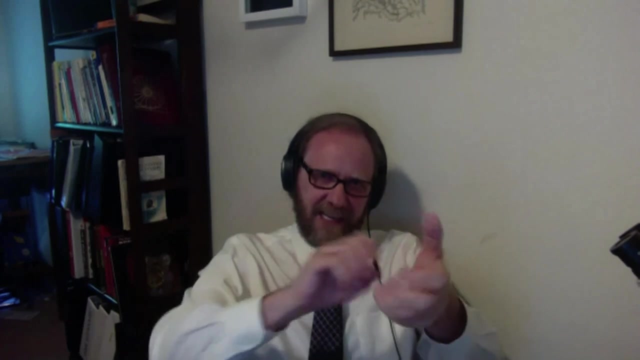 And the second problem is that that's what gets into the museums. As a result, when you're looking at a brittle star that's perfectly preserved, you can't actually see a lot of the morphology that you'd see, Like the inside of the plates, like this, like how the plates articulate on those articulation surfaces. 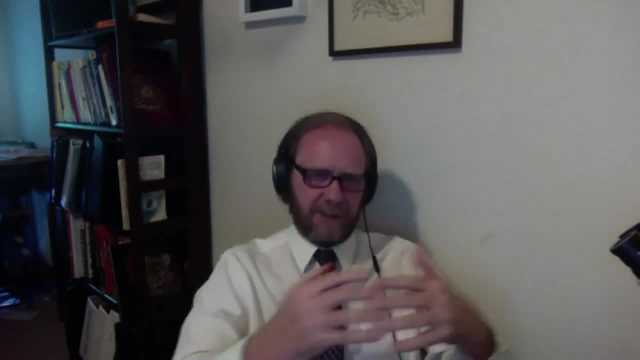 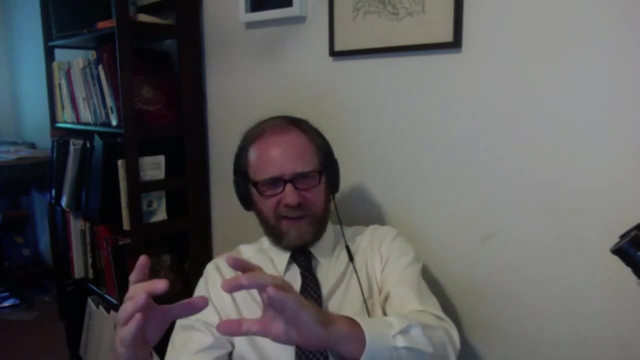 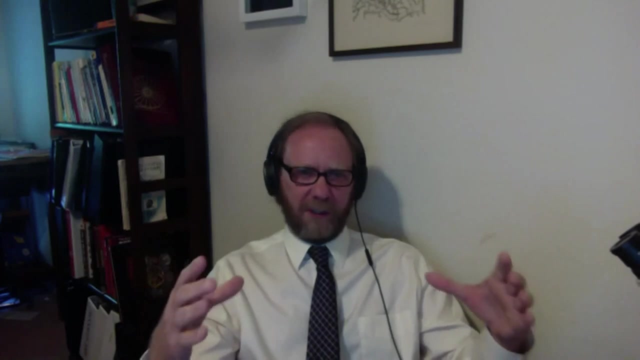 We need the mangled up specimens to be able to see the important things, And so when you only have the really good stuff, you actually can't see. It's sort of like what your advisor told me once upon a time about this croc was so well preserved I couldn't see anything. 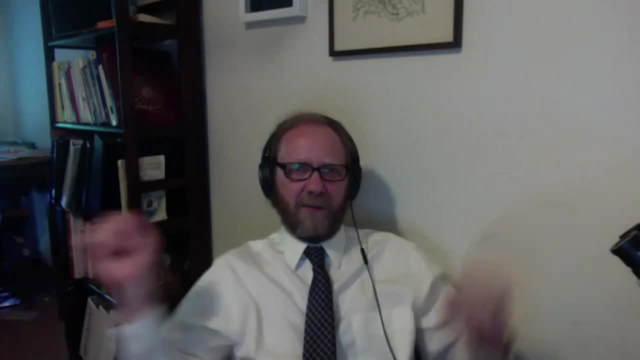 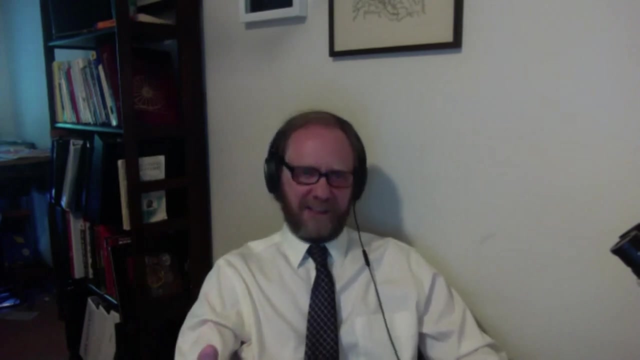 Because all the osteoderms were covering all of it, Yeah, All the important parts, And that's a huge problem. I mean, I've always said with edrio asteroids: give me one really nice, beautiful specimen and 12 that are mangled in various exciting ways, and I'm a happy camper. 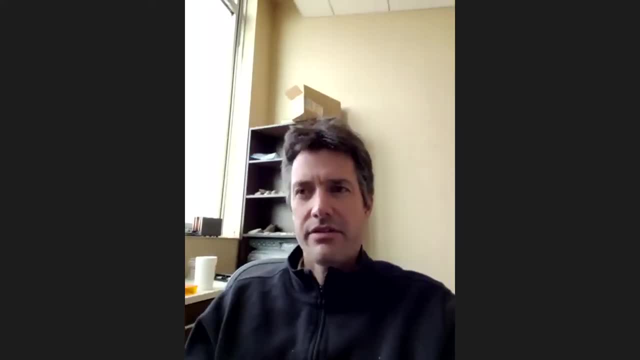 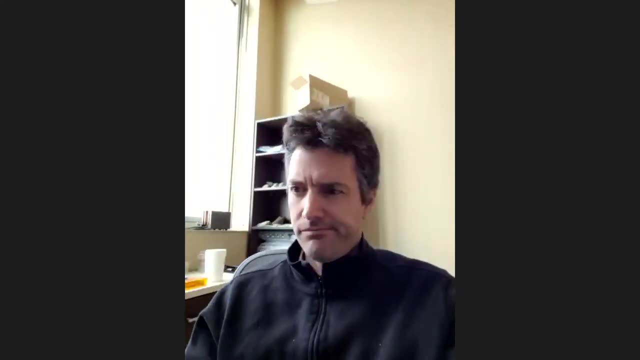 Colin, Yeah, These are very small. I wonder how you do with them. Potentially- I don't know if it's reworking of sediments or you know distribution of these particles, because they might be from very different places than they end up being deposited. 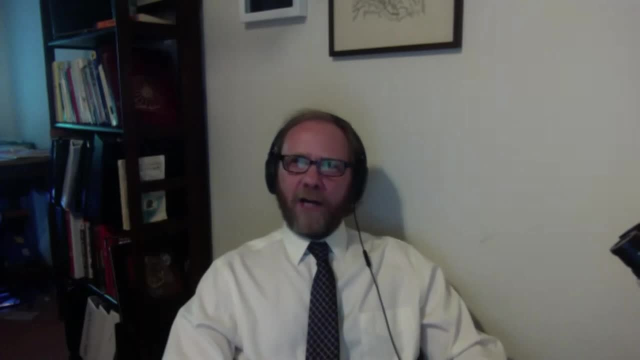 There's actually been a fair bit of work on crinoid disarticulation in the Great Barrier Reef And what we find is that most crinoids, for example, are incorporated into sediment in situ, Which I don't think. I think I find that a little surprising, but in terms of reworking they're certainly not being reworked up section all that much. 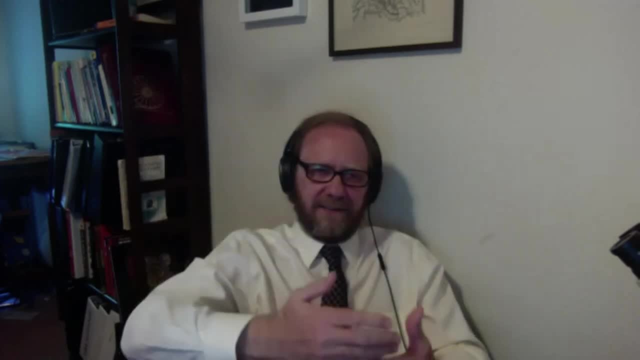 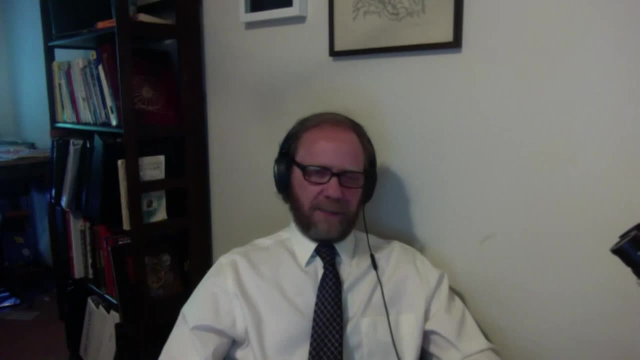 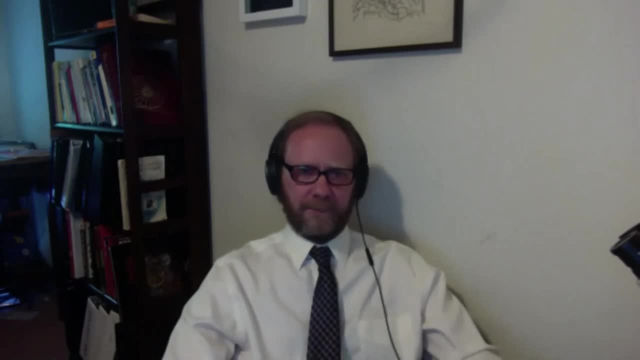 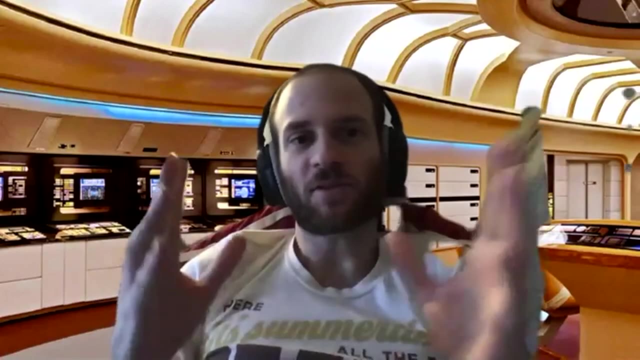 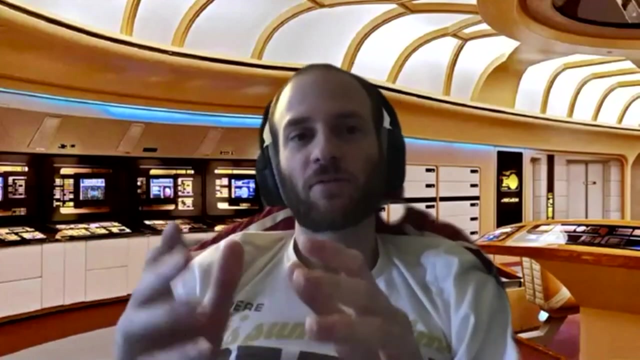 Yeah, Yeah, Yeah Yeah, At least locally here. Hey, Colin, similar question: Have you done any work, Because these are so small and you're getting such a big sample from just one little pile of sediment. have you done any work to see if you sample on one side of the outcrop versus 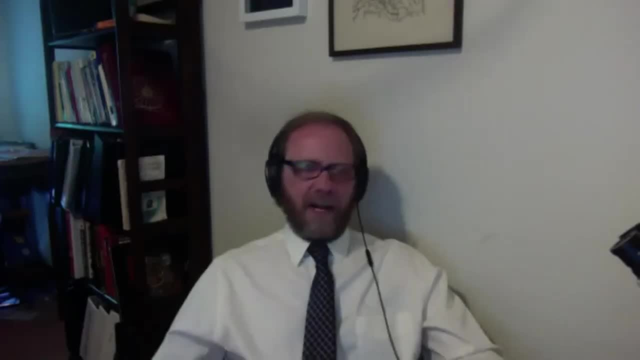 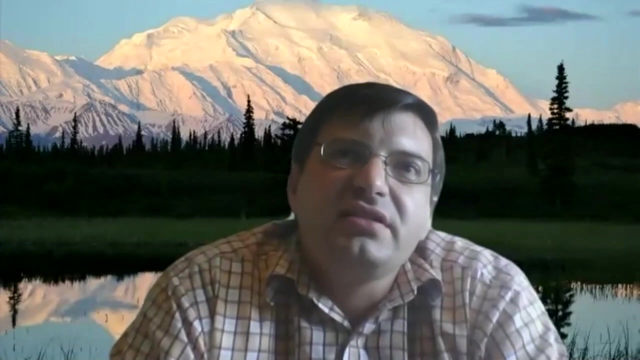 the other if you get different answers. We've done that and you get the same answer. in all, We brought back like 20 bags of this stuff and they're all the same all the same within air bars, Colin. I'm thinking about the imaging problem a little bit more about so all this is based. 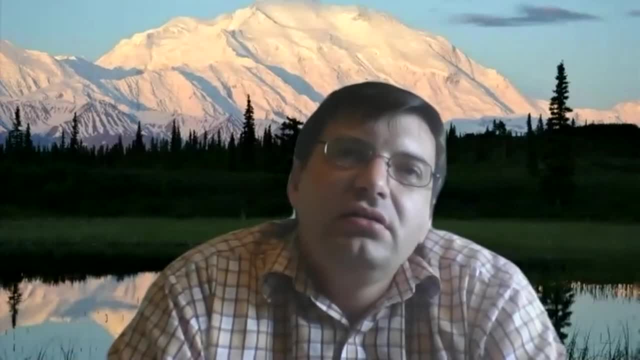 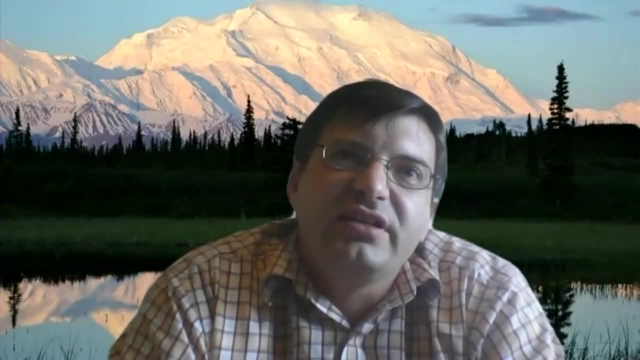 on visual imagery. but if you mapped it chemically, for example, or you went in with other techniques, hyperspectral techniques or something like that, do you think there'd be additional information you could glean by looking at a big pile of this stuff? Would the elements stand out in? 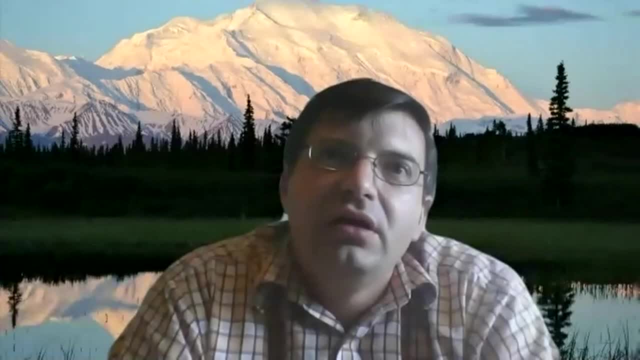 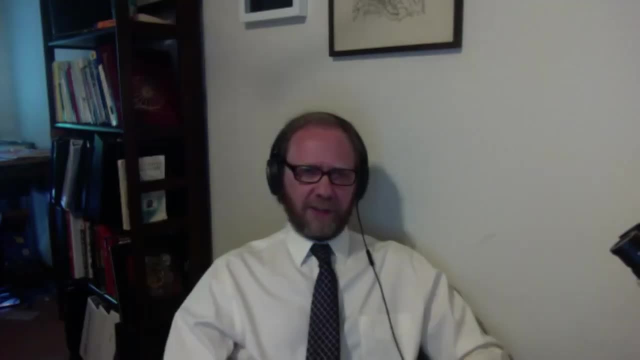 particular ways, or would different species or parts match up in a way that lets you One would think that things, that all the echinoderm parts might group together, but you're also, you also have to concern yourself with. you know crinoids. have you know more parts than 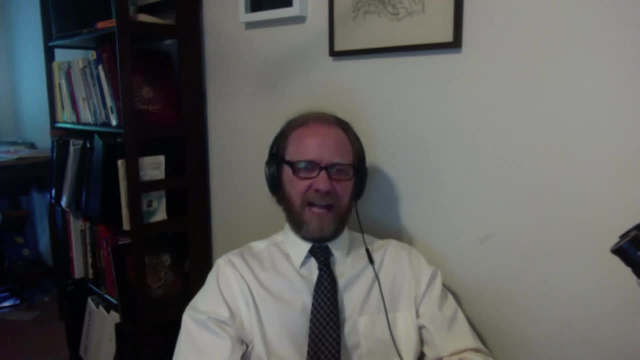 brittle stars and they are more numerous, And the localities in brittle stars and have pieces that are of the same basic size fraction. So you're going to get a lot of swamped signals there. I would imagine that. I mean if you fingerprint them chemically, I'm sure the echinoderms would. 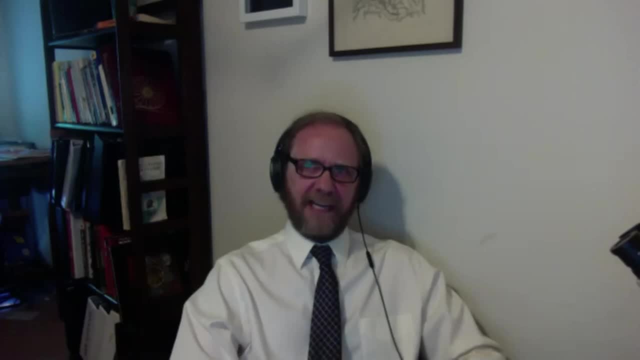 be distinctive in that they start out as magnesium calcite, and the only other magnesium calcites in there would be maybe the bryozoans and the brachiopods, which are pretty common in there. There's probably ways to do it, but again, you've still got to figure out what you're seeing and 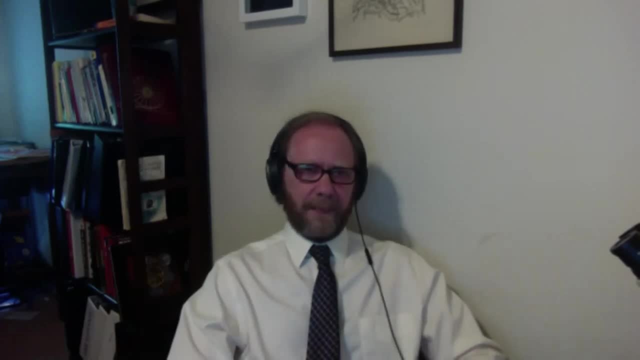 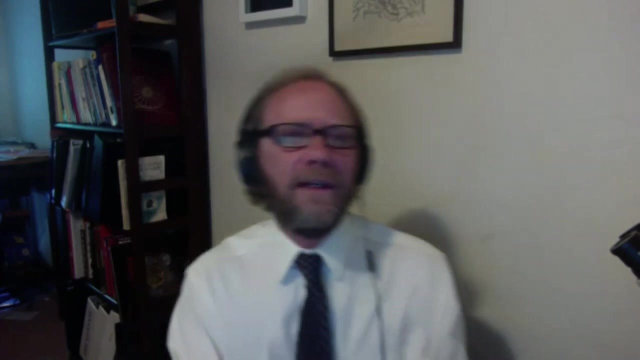 that's the biggest problem. Okay, well, I guess that's it, and thank you all for coming. Thanks for watching and we'll see you next time. Thank you.